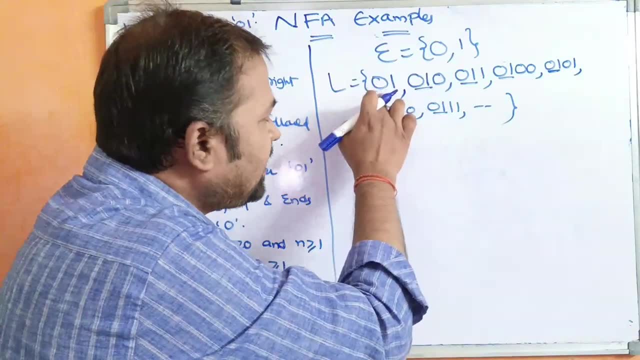 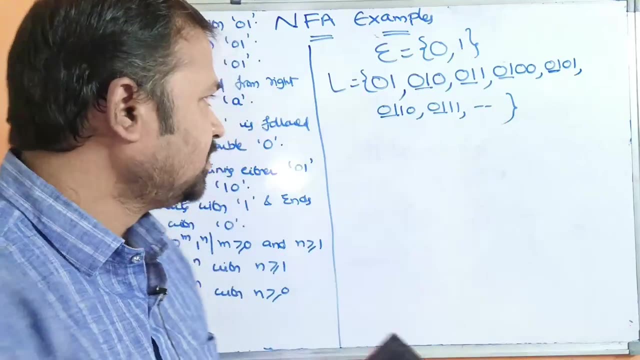 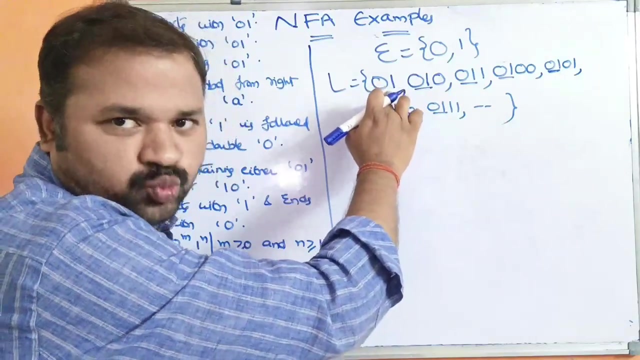 to construct the NFA. So here the length of the minimum string is 2.. So we require 2 plus 1, 3 states. Why? Because here what is the minimum string? here The minimum possible length here is 2.. So 2 means we require 2 plus 1. So we require 3 states. So here we. 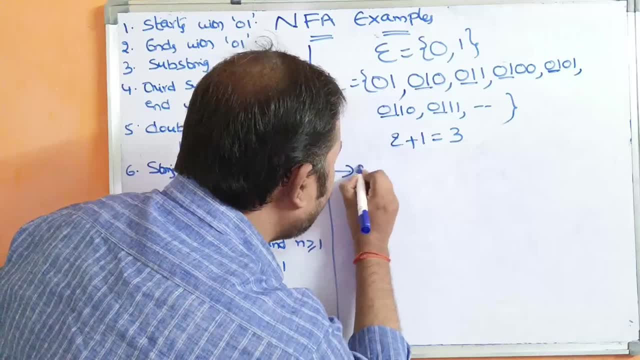 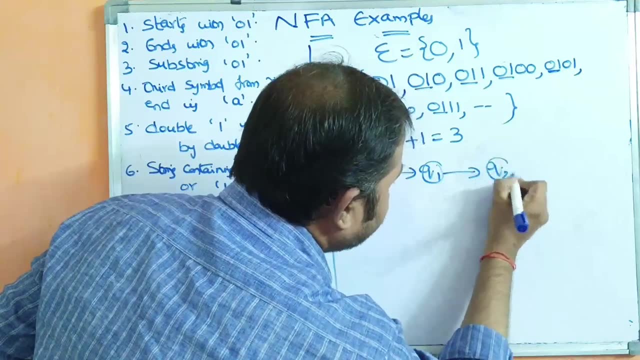 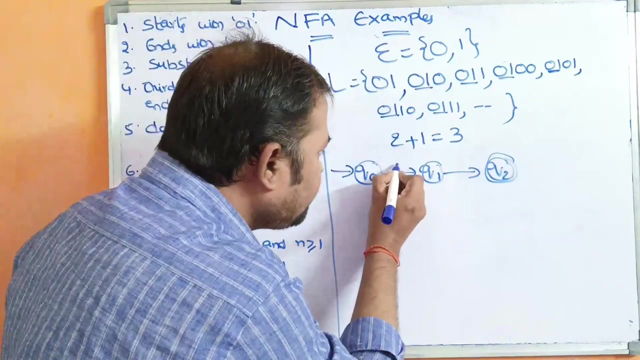 require 3 states. Let the first state is q0.. Second state is q1.. Third state is q2.. So this is the final state where q0 is the initial state. So here we have to apply 0, 1.. So 0. 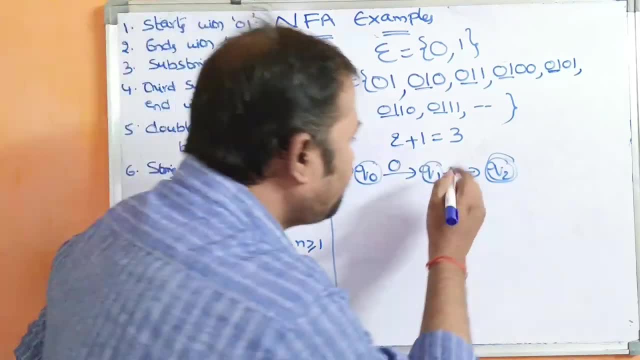 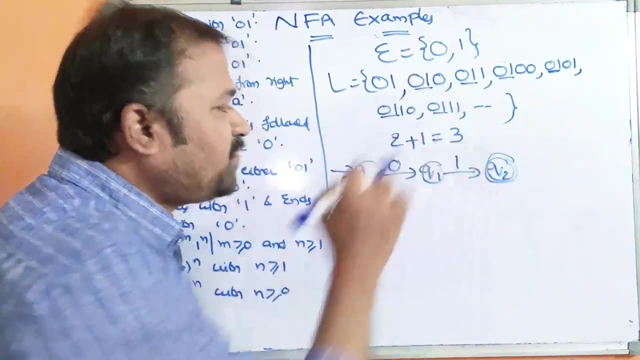 on q0 means we will move to q1 state. 1 on q1 means here we are moving to q2 state. Here the string starts with 0, 1.. After that we can have any number of 0s and 1s, So here: 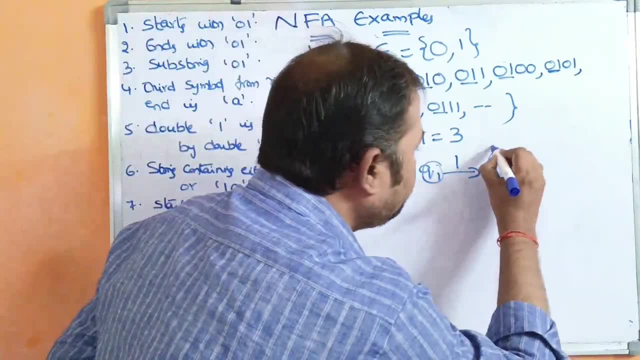 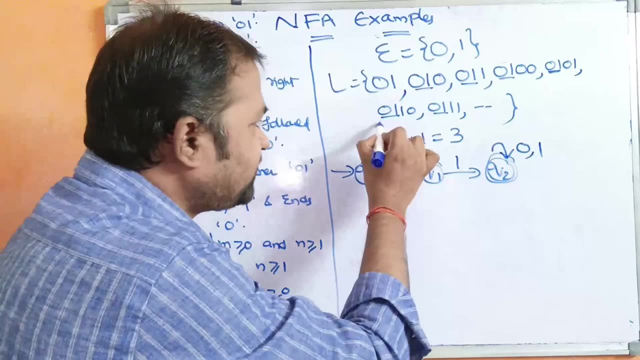 we have any number of 0s and 1s. So on q2, just apply the self loop, So 0, 1.. Let us take any string, Let us consider this one: 0, 1, 1, 0.. So let us apply 0. So we will. 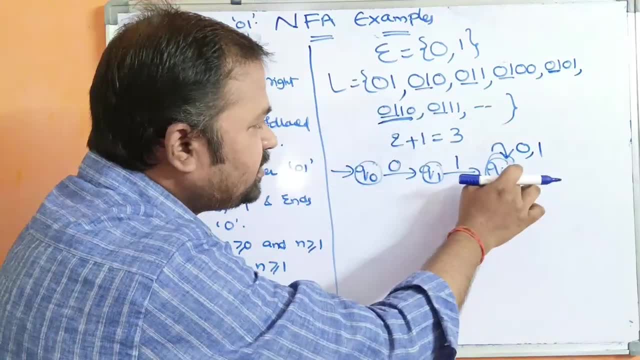 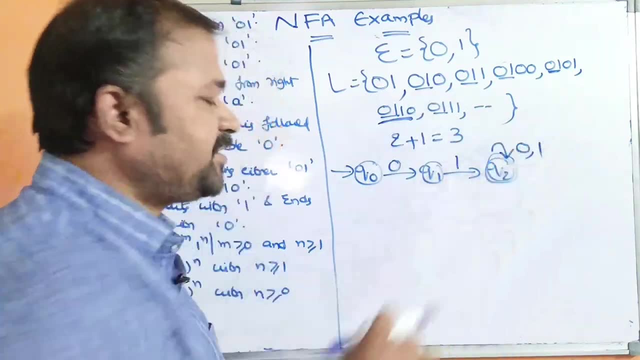 move to the q1 state. Now let us apply 1.. We will move to the q2.. Next, let us apply 1.. So we will be in q2 state only. Let us apply 0.. So we will be in q2 state only So. 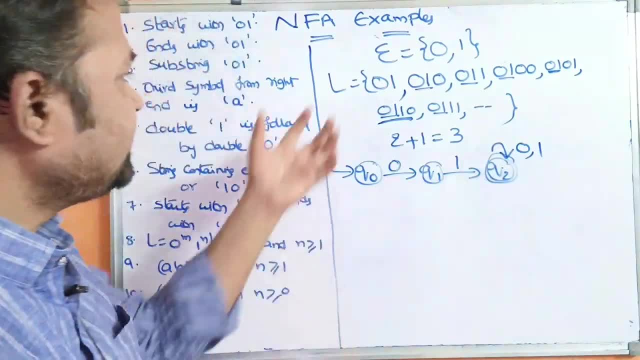 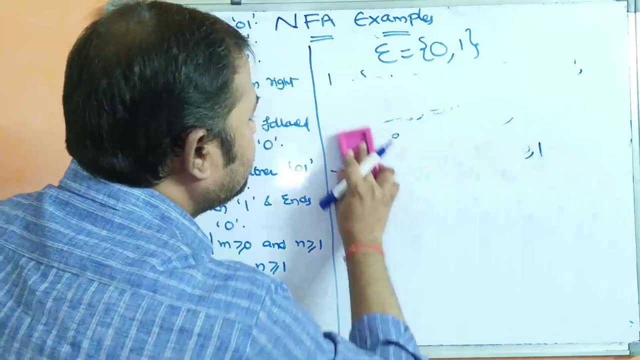 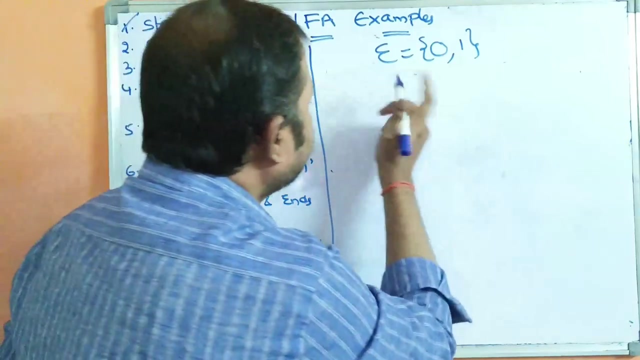 q2 is nothing but the final state. So in this way we can design NFA for the string starting with 0, 1.. Now let us see the second problem. So what is the second problem? Strings ending with 0, 1.. So strings ending with 0,. 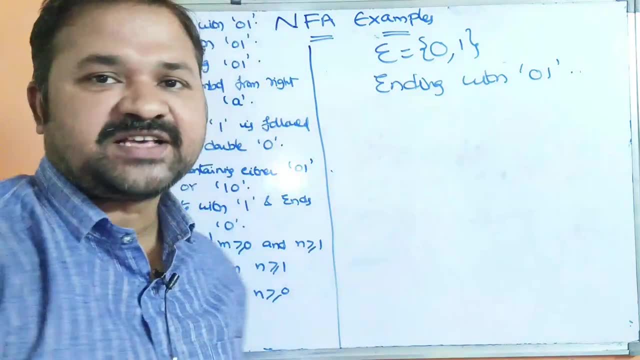 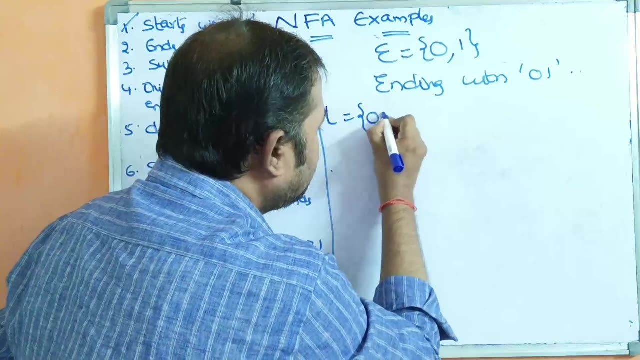 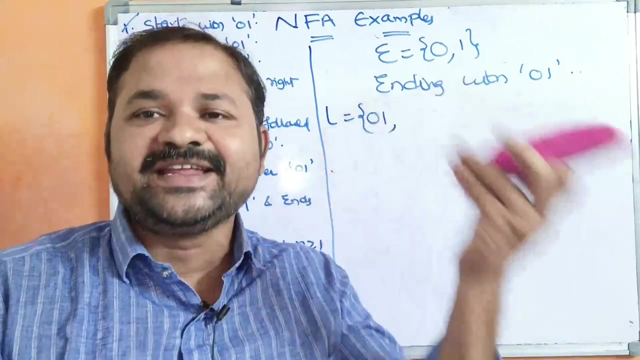 1.. So first let us construct the language. Let us write the language. l is equal to 0, 1.. So strings ends with 0, 1.. So before 0, 1, we can have any number of 0s and any number. 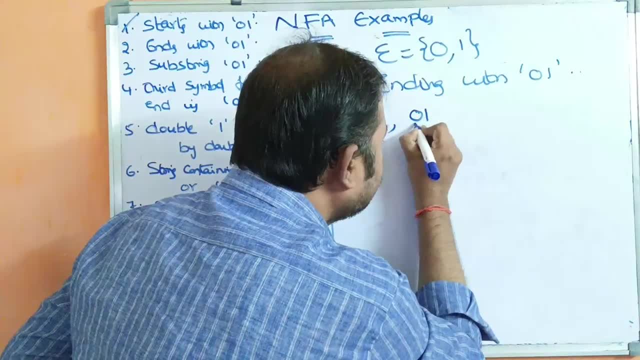 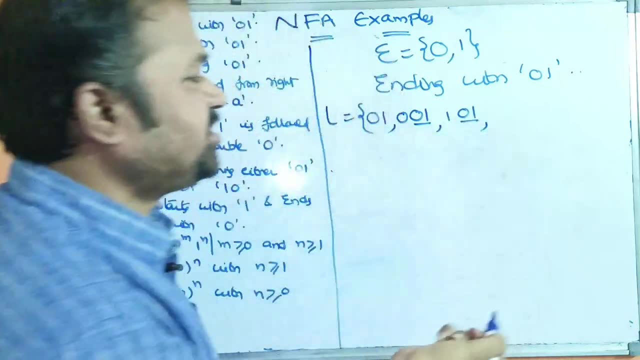 of 1s, So strings ending with 0, 1.. So before 0, 1, we can have any number of 0s and any number of 1s, So there is no restriction on that. So 0, 1.. Let us take string of 2, length. 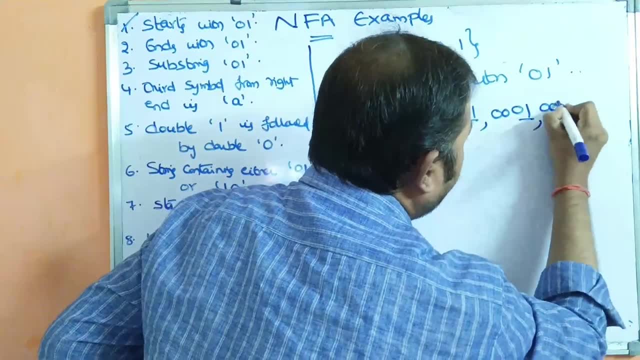 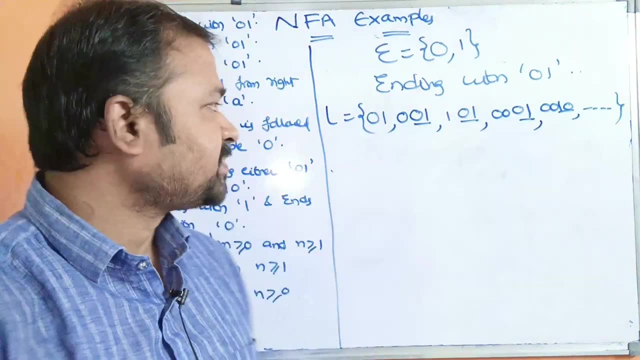 of 2.. So 0, 0.. Next 0, 0, 1, 0.. So likewise we can have n number of 0s and n number of strings. Now let us design the NFA Here. the minimum string is 0, 1.. So length of the. 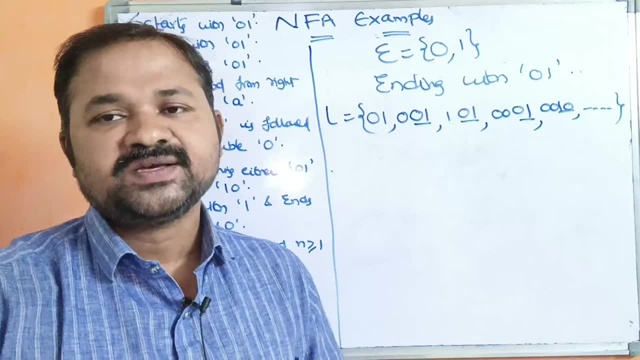 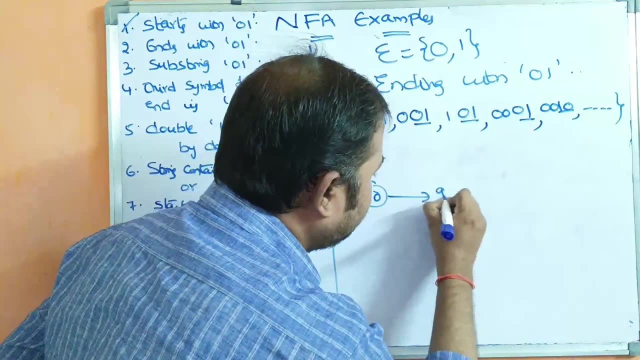 minimum string is 2.. So here the length is 2. So we require 2 plus 1, 3 states. So the possible states here are q0, q1, q2.. So q0 is the initial state, whereas q2 is the final. 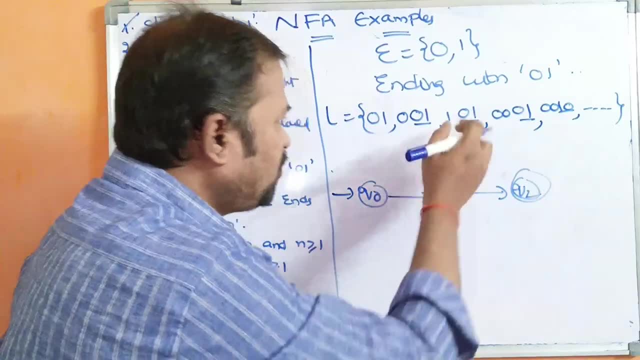 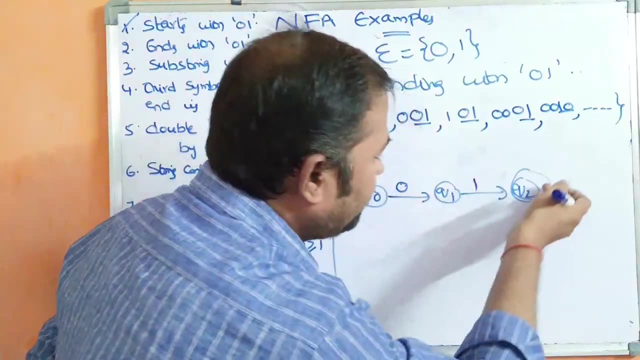 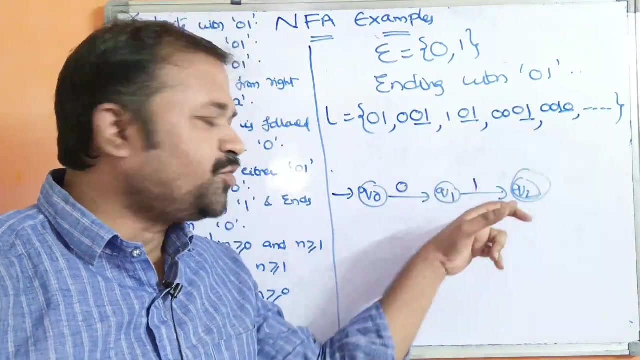 state. So here we are moving to q1 state. Let us apply 1 on q1.. So here we are moving to q2 state. Next, here here the strings are starting, ending with 0, 1.. So before 0, 1, we can have. 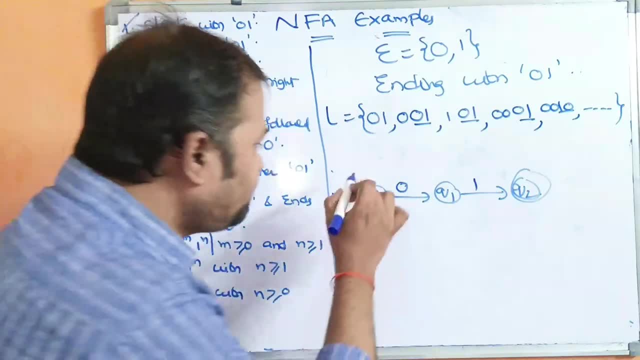 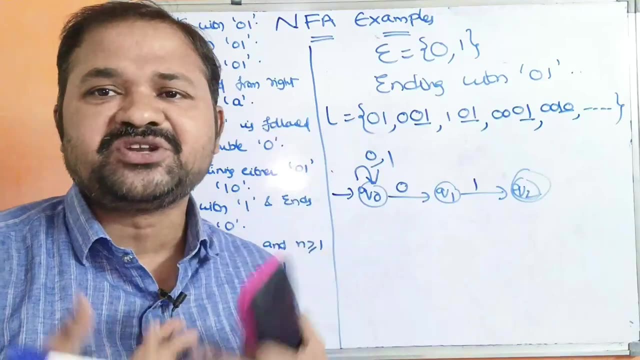 any number of 0s and any number of 1s. So, simply, we can apply the self loop. We can apply the self loop, So before 0, 1, we can have any number of 0s and any number of 1s. 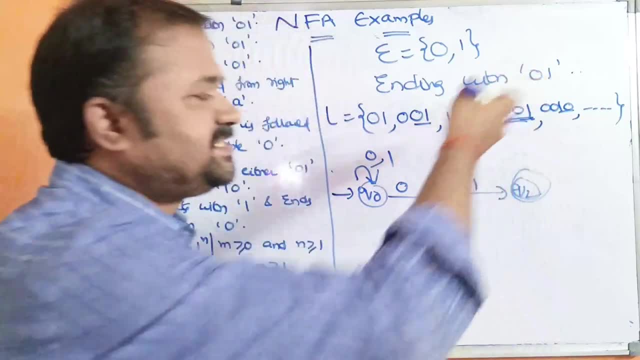 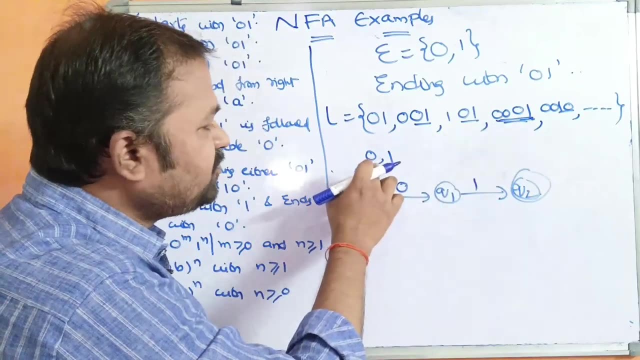 So let us take one string. Let us take this string 000.. So 000, 1.. So 000, 1 means. so let us apply 0 on q0.. So we will be at q0 only Next. let 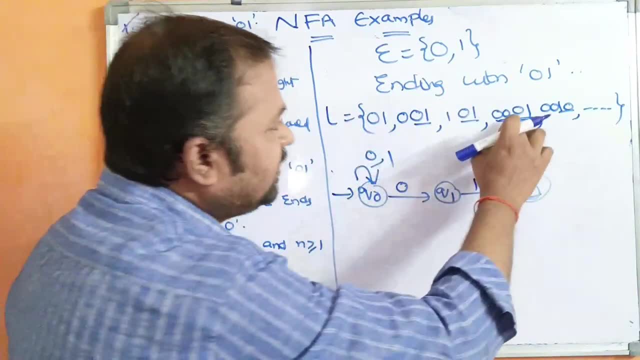 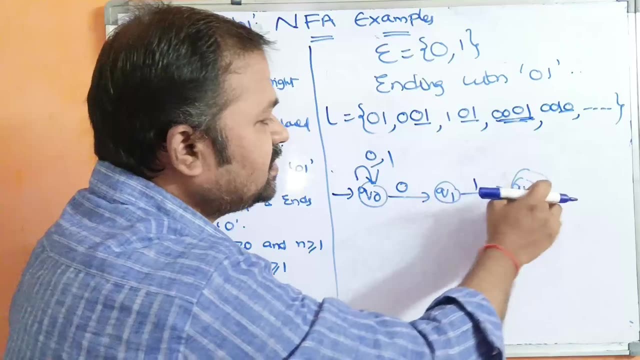 us apply 0 on q0.. We will be at q0 only. Next 0, 1.. Let us apply 0 on q0.. So we will move to the q1 state. Now. let us apply 1 on q1.. So we will move to the q2 state. So q2 is. 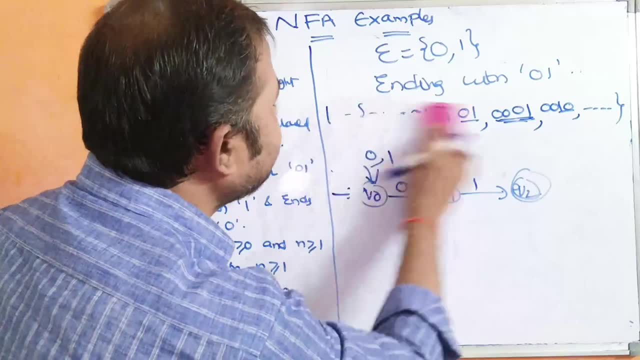 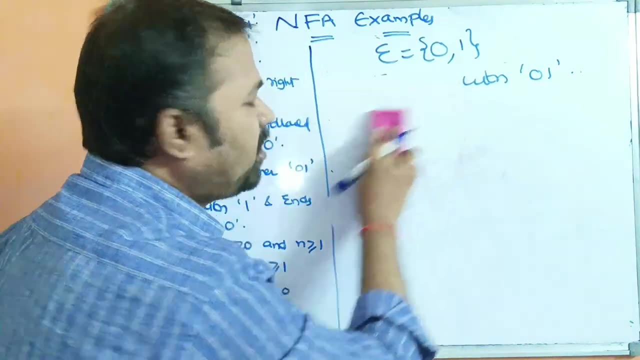 nothing but final state. So in this way we can design NFA for ending with: So it may be 0,, 1.. So it may be 0, 1, or ab or xy. So for all the problems the solution is same, only Now. 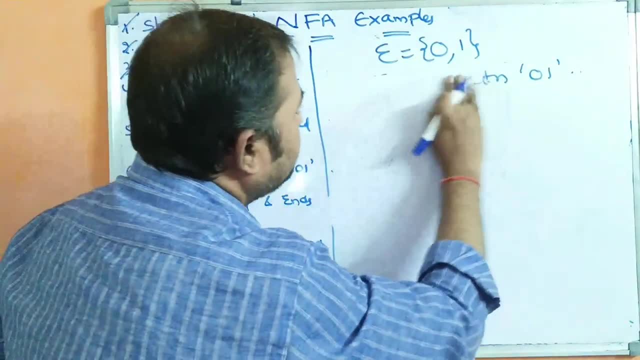 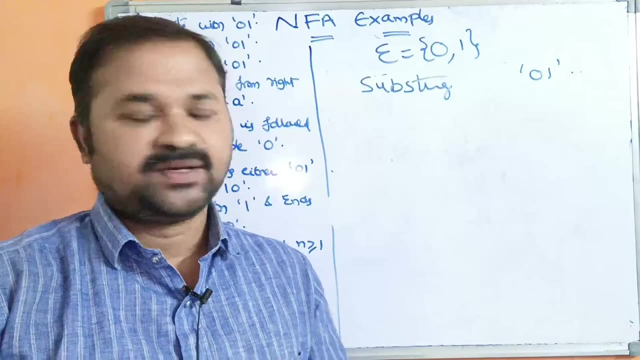 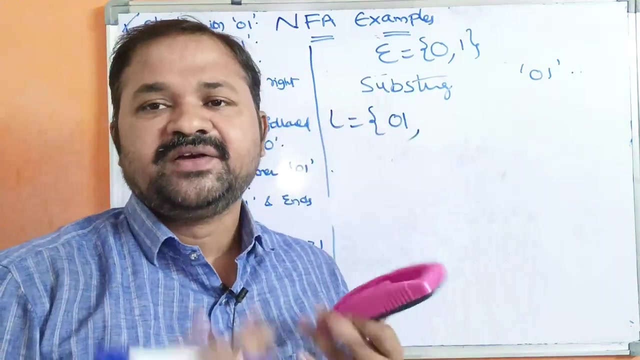 next example: substring 01.. So we have to design NFA for the strings whose substring is what 01.. So let us design the, let us write the language So 01.. So here, before 01, we can have any number of 0s and 1s. After 01, also we can have any number of 0s and. 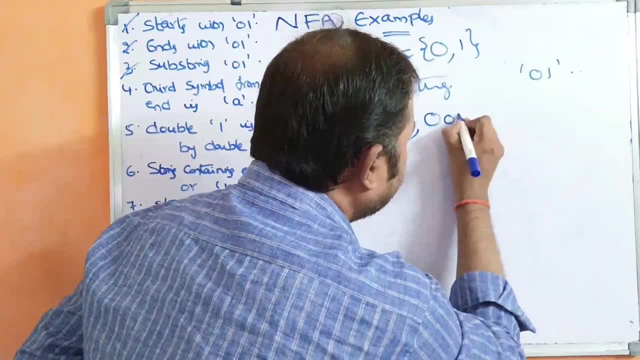 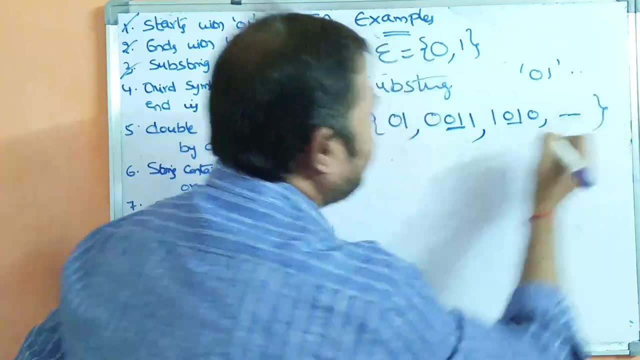 1s. So there is no restriction on that. So 0, 0, 1, 1.. 1, 0, 1, 0.. So likewise, we can write a number of strings. Okay, So here the minimum possible, here the minimum string. 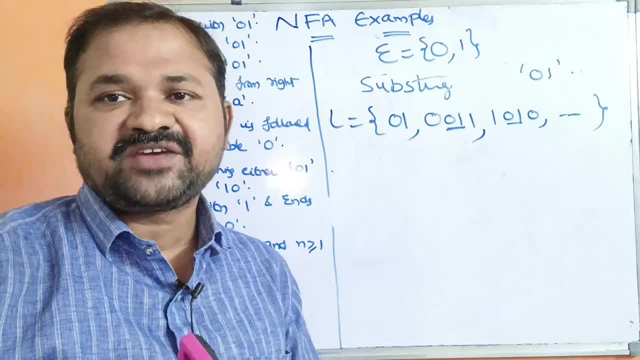 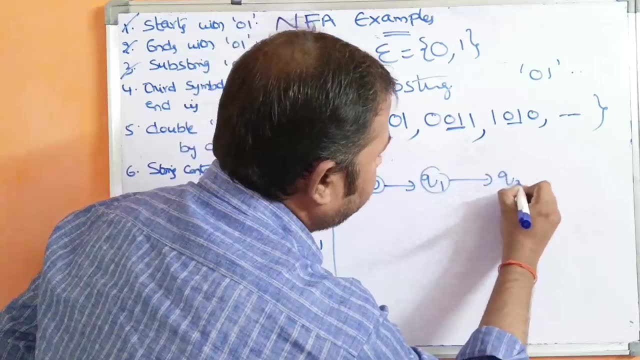 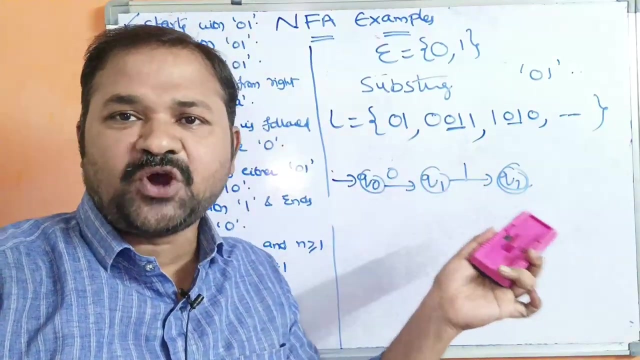 is 01.. So this minimum string length is 2.. So we require 2 plus 1, 3 states. So the 3 states are q0, q1, q2.. So let us apply 01.. Here is the substring. Substring is 01.. So before 01, we can have any number of 0s and 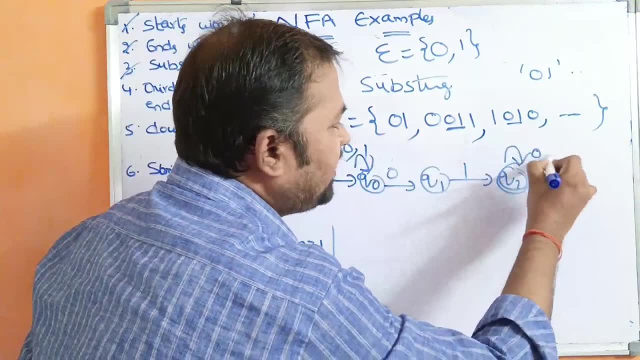 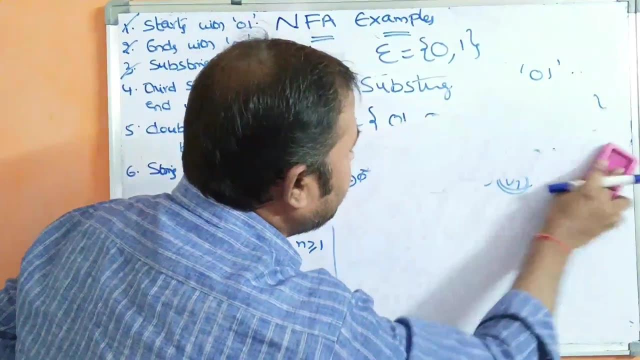 1s, So after 01 also we can have any number of 0s and 1s, So simply apply the self-loop. Okay, So in this way we can design for design the NFA for the substrings. Now let us see. 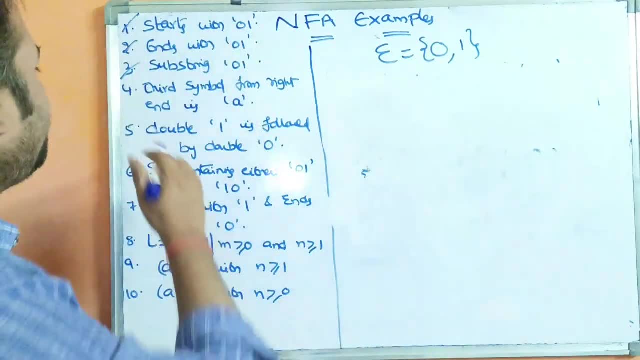 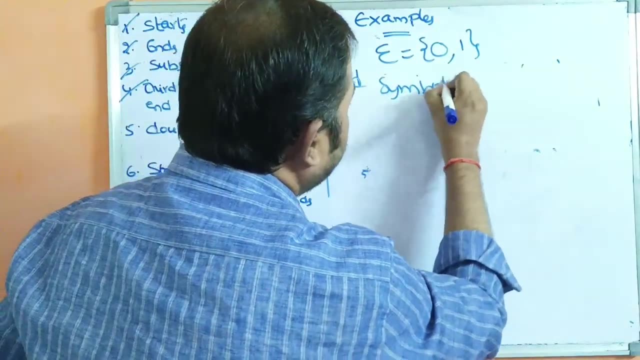 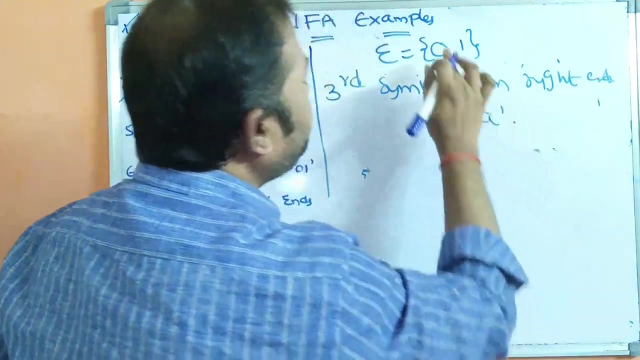 the next example. The next example is: third symbol from the right end is a. So third symbol, third symbol from the right end is a. So third symbol from the right end is a. So third symbol from the right end is a. Here the input alphabet contains 2 symbols. They are a, b, So here. 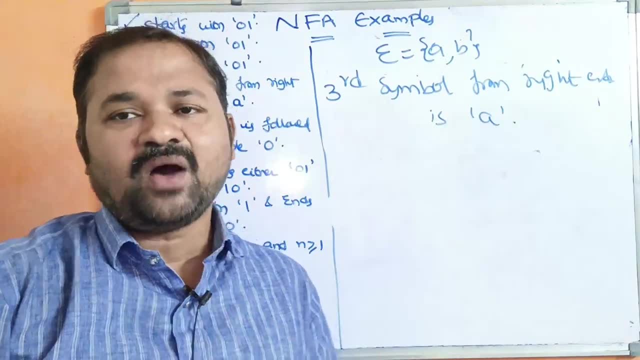 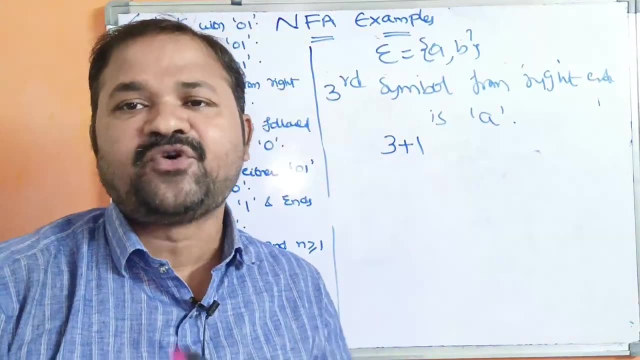 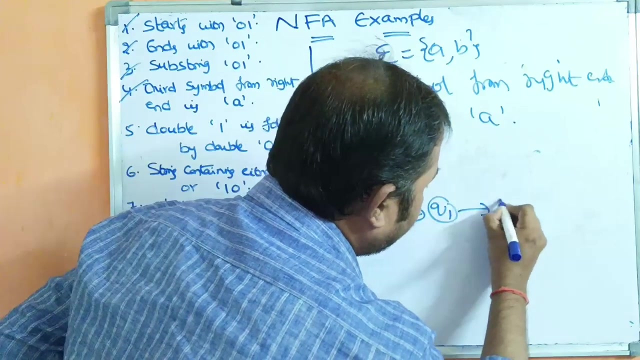 third symbol from the right end is a. So we have third symbol means 3 symbols. So here we must require 3 plus 1.. We must require 4 states. So first let us draw some skeleton. So 4 states, So q0,, q1,, q2.. 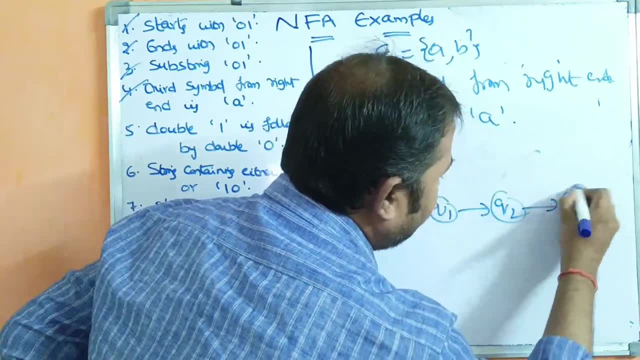 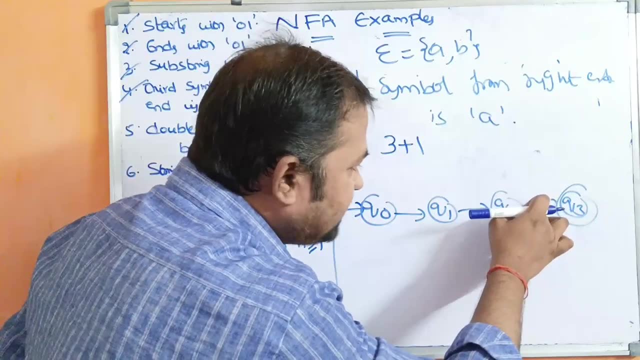 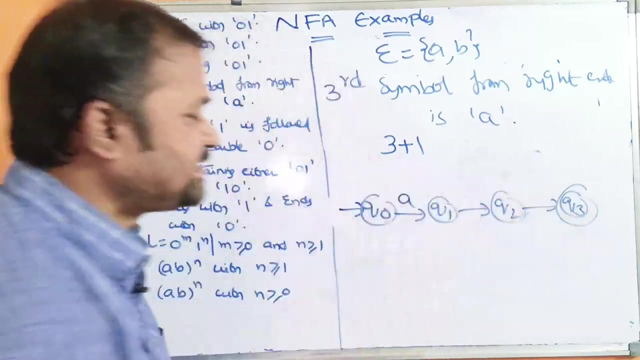 q2, q3.. So q3 is nothing but final state, q0 is nothing but initial state. Third symbol from the right end is a. So this is the rightmost symbol, Next to second rightmost, one third rightmost. So third symbol from the right end is a. And after that, if we apply, we can. 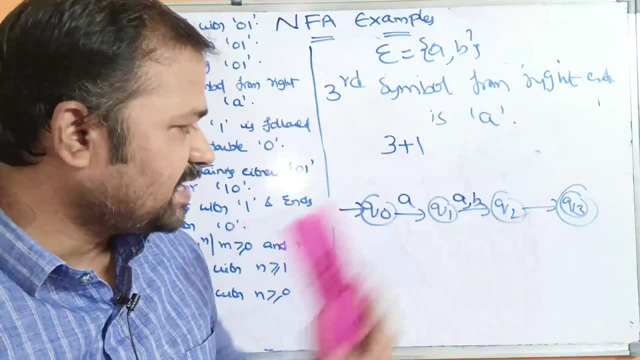 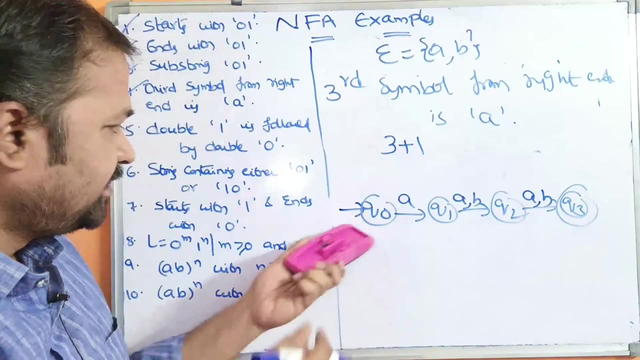 apply a, b and q1.. If we apply a, b and q1, then we will go to the q2.. Likewise, we can apply a, b and q2.. So we will go to the q3 state Next here, before this third symbol from the right end. 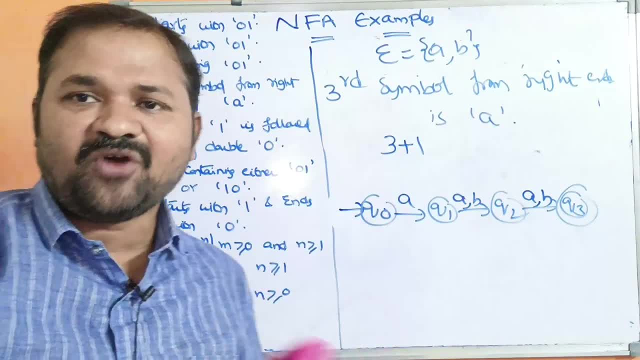 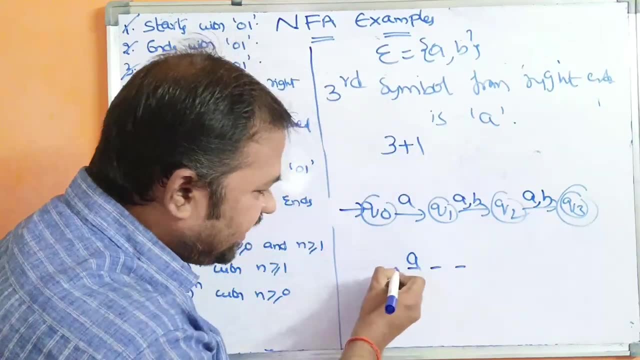 is a, So before this we can have any number of a's and b's. So here, third symbol from the right end is a, So before this a, we can have any number of a's and b's. There is no. 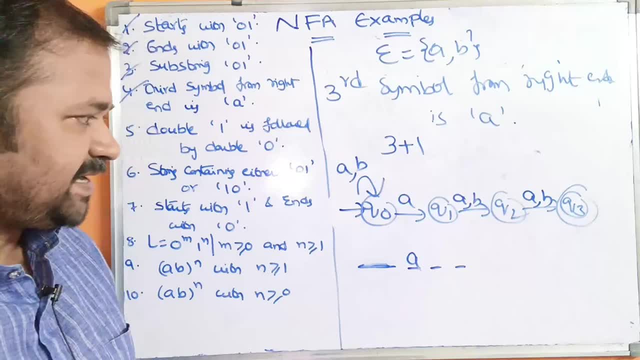 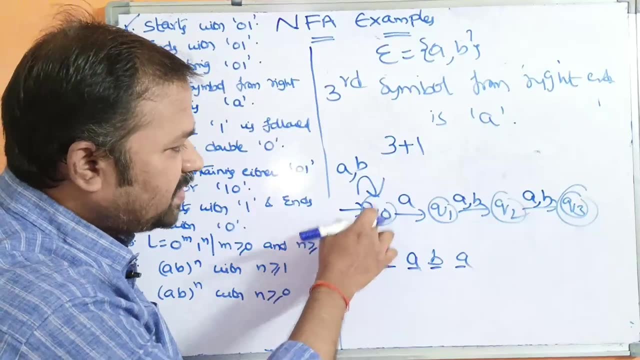 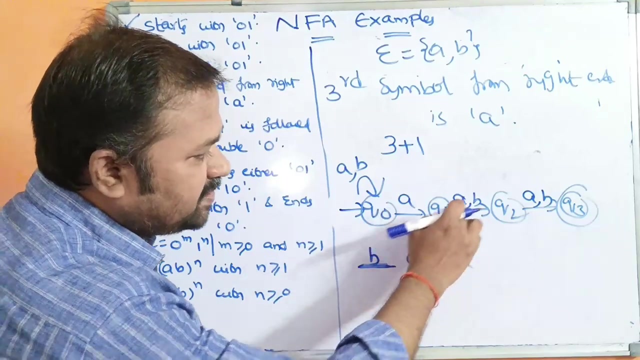 restriction on that. So we can apply the self-load a, b, Let. the string is like this: b a, b, a. Now let's apply q0.. Until we apply q1, we will be at q0 only. Let us apply a on q0.. 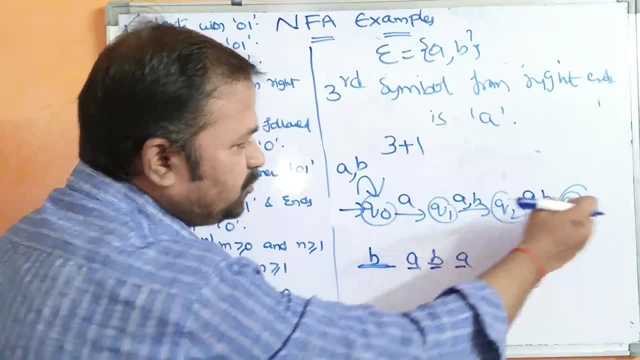 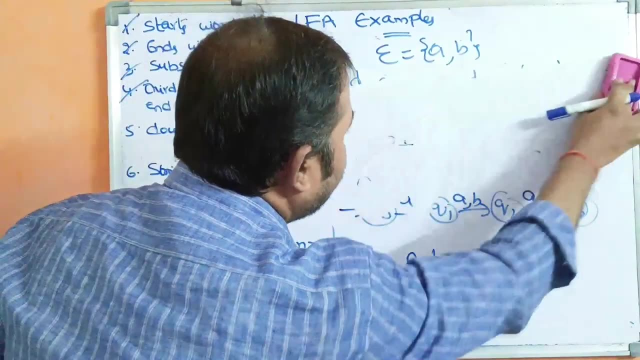 We will move to the q1 state. Let us apply b on q1.. We will move to the q2 state. Let us apply a on q2.. We will move to the q3 state. q3 is nothing but final state. So in this, 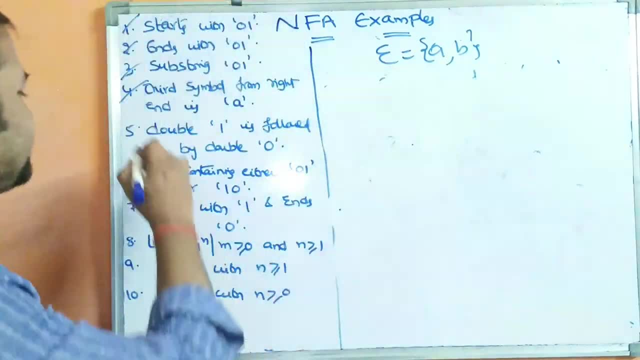 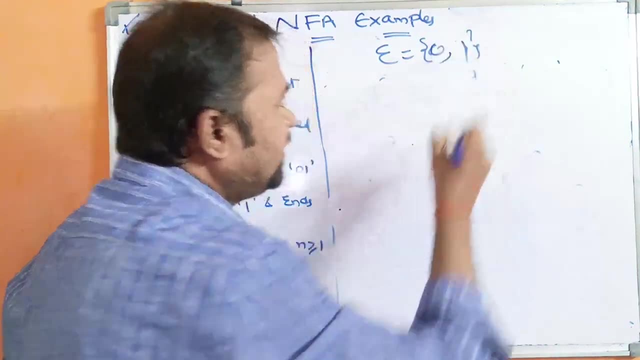 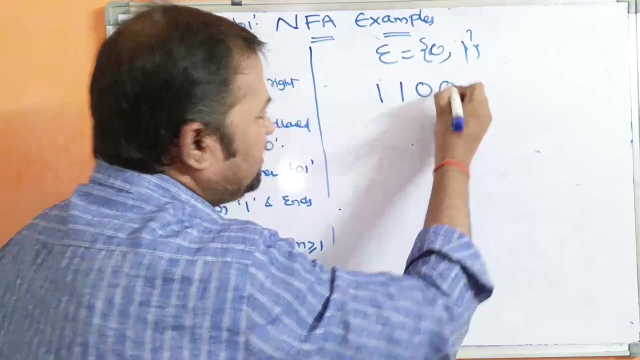 way we can design the DFA. Now let us see the next example. Double 1 is followed by double 0. So here the alpha and 1.. So here, directly, the problem is given: Double 1s is followed by double 0. So 1, 1, 0, 0. 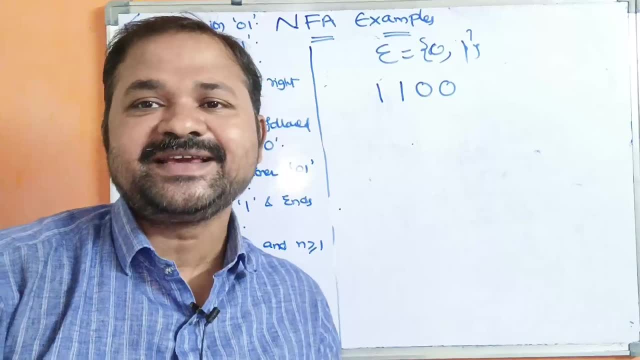 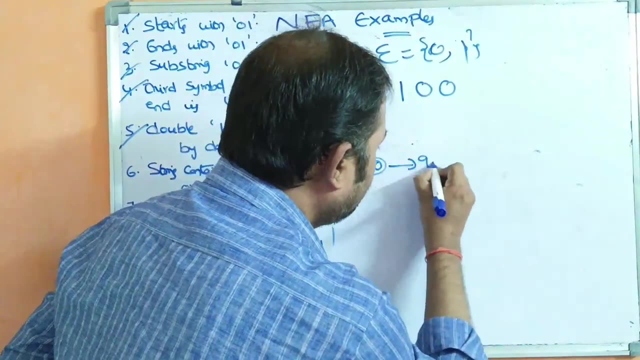 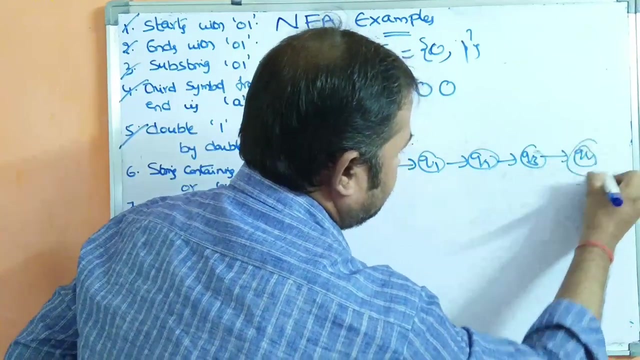 is the minimum string. So here the length of the minimum string is 4.. So 4 means we require 5 states. So we require 5 states. So Q naught Q 1,, Q 2,, Q 3,, Q 4, 5 states. So Q 4 is the final. 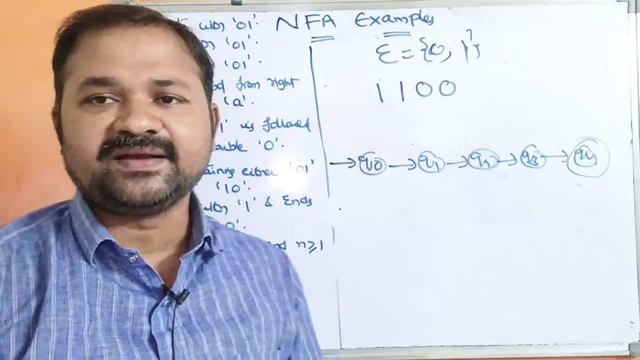 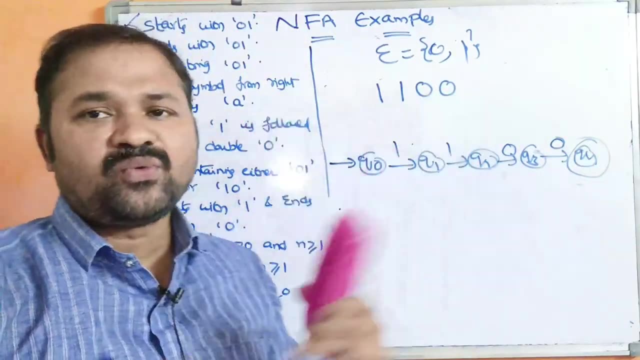 state Q, naught, is the starting state. So double 1 is followed by double 0. So 1 1 0 0.. And before 1 1 0 0, we can have any number of 0s and 1s. There is no restriction on that. 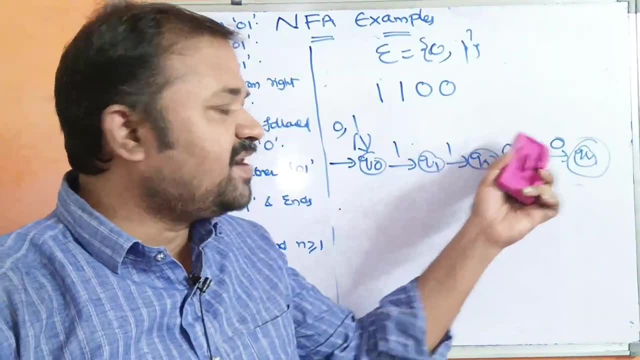 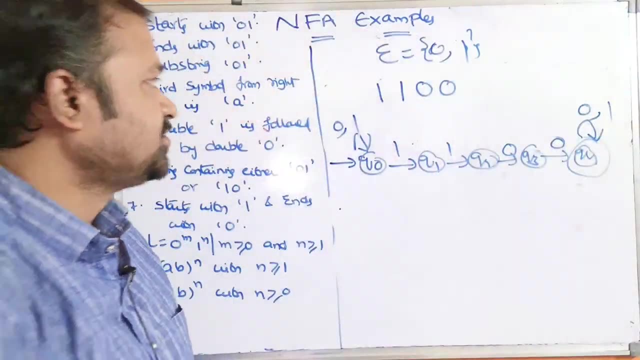 So let us apply the self-rule: 0: 1.. After double 1, double 0, we can have any number of 0s and 1s. There is no restriction on that. So let us apply the self-rule, So in this way we can solve the. 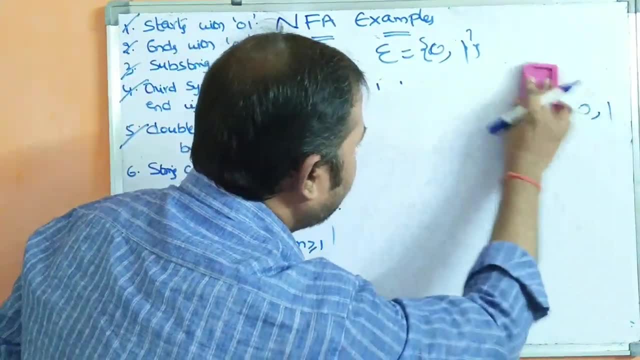 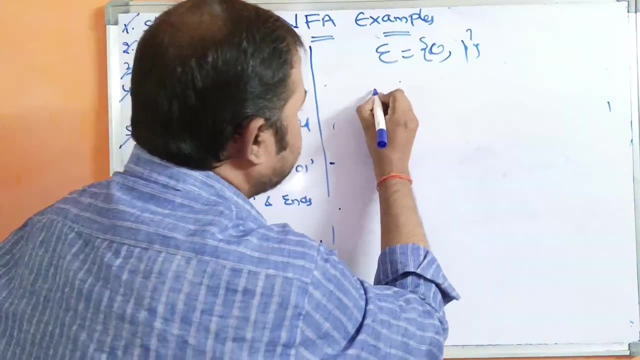 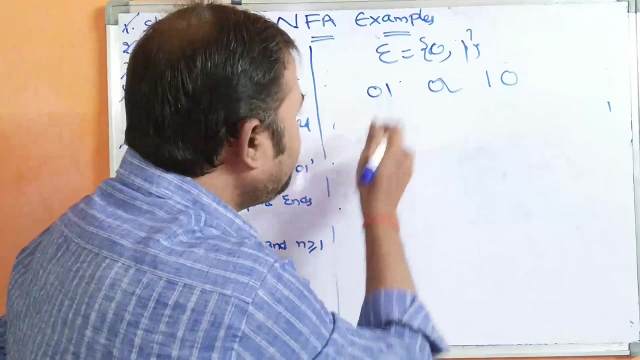 problem. Now let us see the next example. So what is the next example? String containing either 0, 1 or 1, 0.. So string must contain either 0, 1 or 1, 0.. 0, 1 or 1, 0.. So here for 0, 1, we require how many states 0, 1 means length is 2.. So 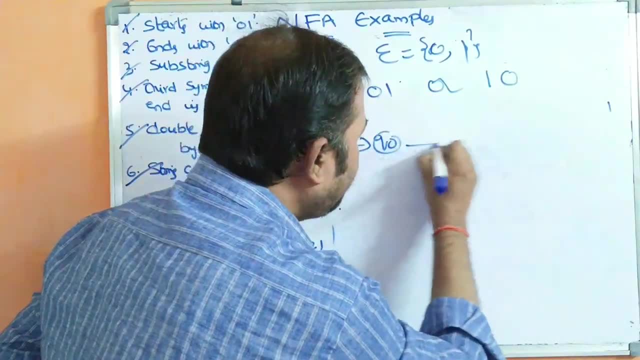 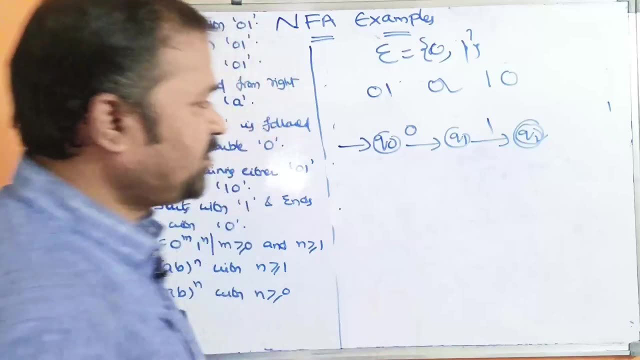 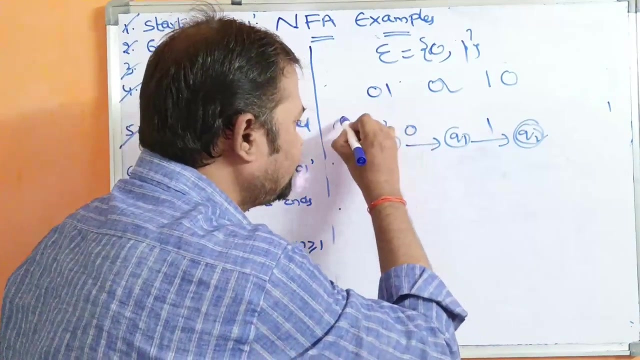 2 plus 1 means we require 3 states, So Q naught Q 1, Q 2.. So string contains 0, 1.. So 0, 1.. So before this 0, 1, we can have any number of 0s and 1s, So there is no restriction on that. 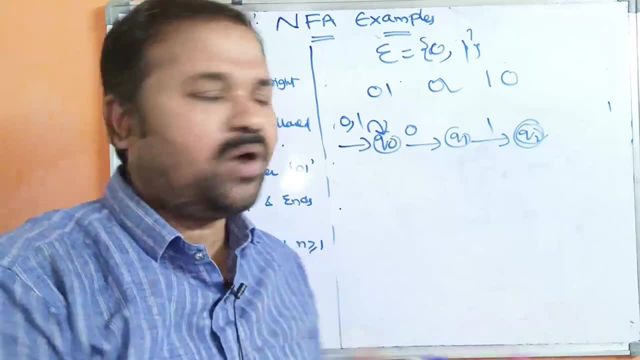 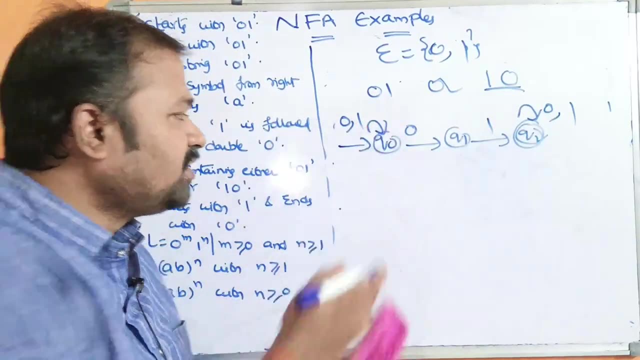 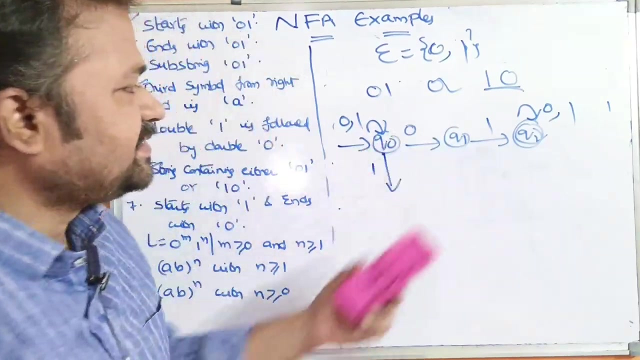 So 0, 1.. So after 0, 1 also, we can have any number of 0s and 1s. Or what is the second string, 1, 0.. For 1, 0, let us write the transitions like this: So 1,. if we apply 1,, then we will go to. 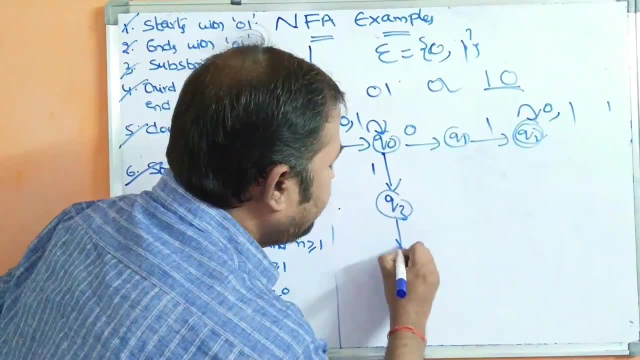 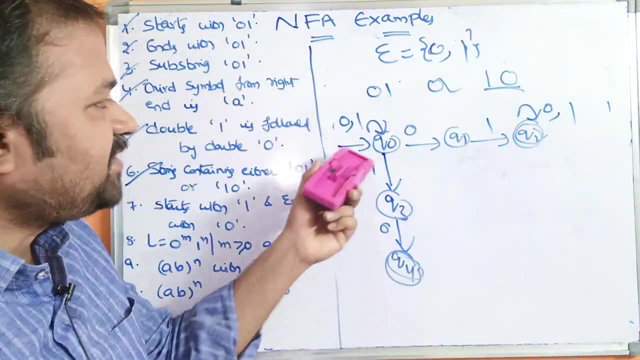 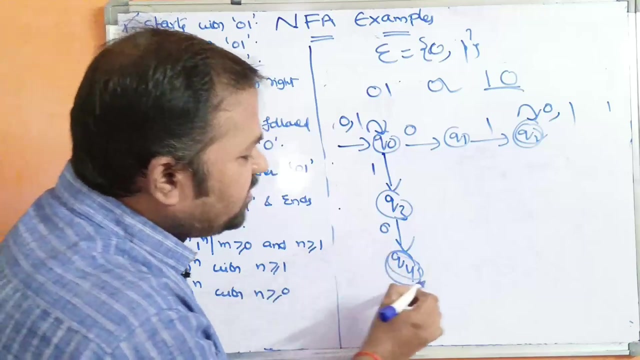 Q 2 state is over Q 3.. Next, if we apply 0,, then we will go to the Q 4 state. Here Q 4 is the final state for this transition: 1: 0.. So string starts with either 0, 1,, 0, 1 or 1: 0.. So after 1: 0, we can have any number of 0s and 1s. 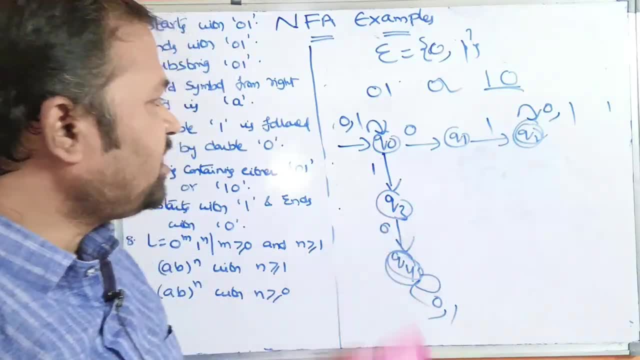 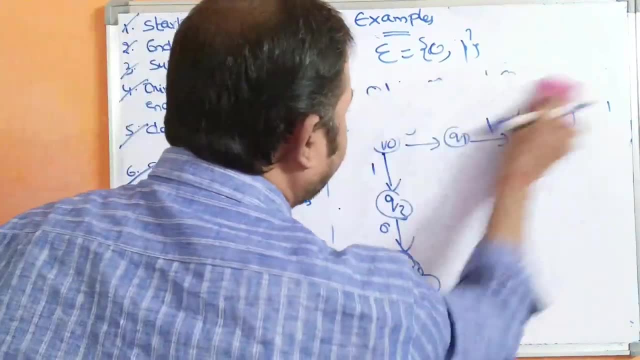 So there is no restriction on that. So this is the NFA, which accepts the strings containing either 0, 1 or 1- 0.. So in this way we can draw the NFA. Now let us see the next. 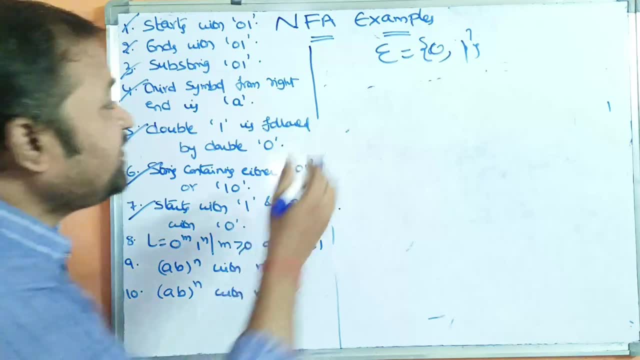 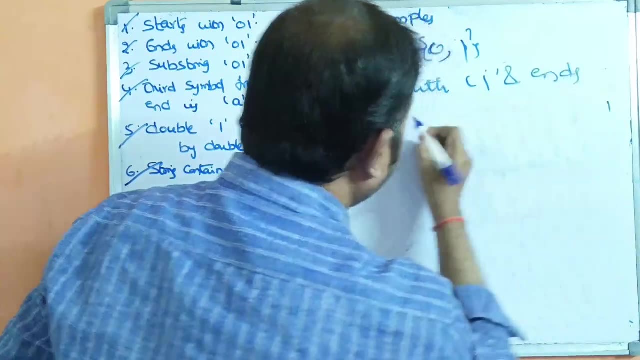 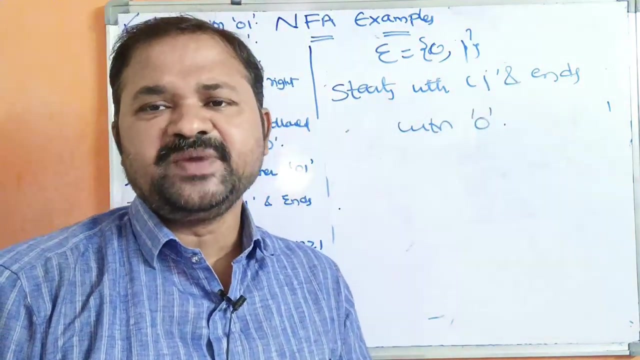 example, Starting with 1 and ends with 0. So starts with 1 and ends with 0. So here the minimum string is what? 1: 0.. So 1: 0 means length is 2.. So the possible number of states are 2 plus 1,. 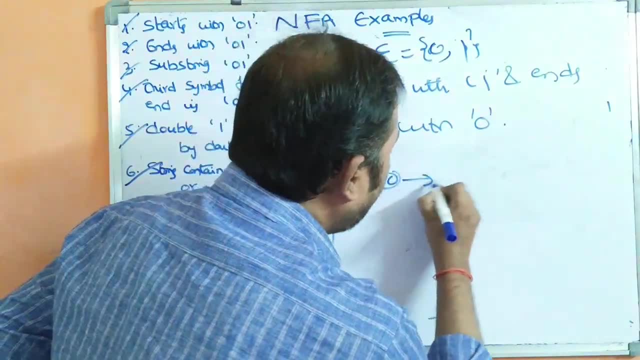 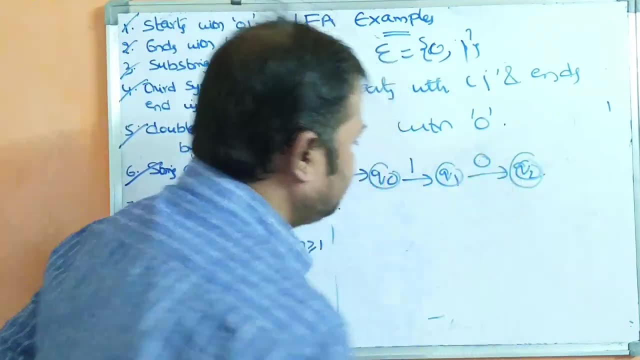 3. So we require 3 states. So Q naught Q 1, Q 2.. So string starts with 1,, ends with 0.. Starts with 1, ends with 0.. Here, after the 0,. 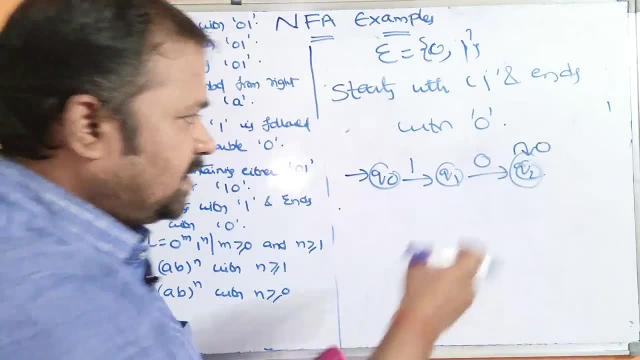 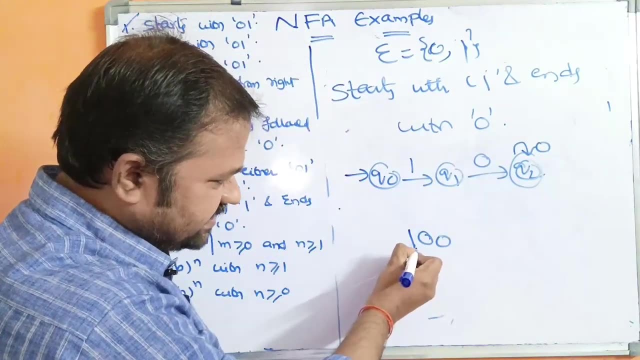 we can have any number of 0s, There is no problem Here. we may have 0 here also. So 1 0 0, 1 0 0.. So here the string starting with 1, ends with 0. So if we apply 1,, then we will move to the Q 1. 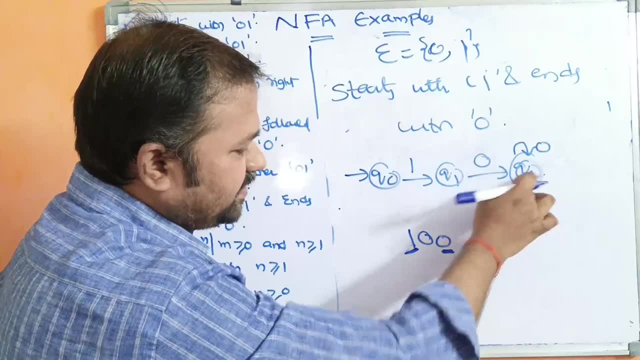 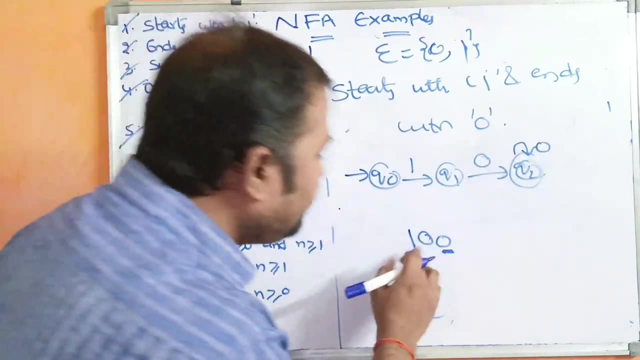 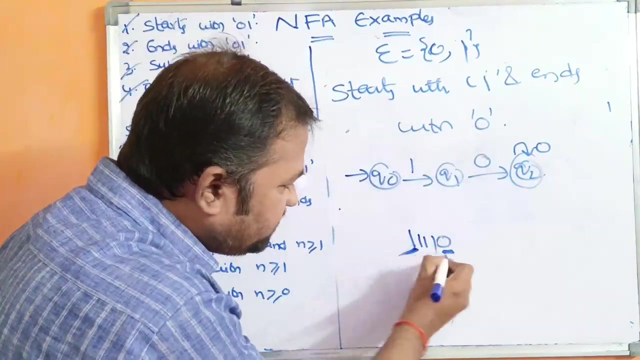 state. Next: if we apply 0, we will go to the Q 2 state. Next, if we apply 0 on Q 2, we can have any number of 1s. Here the constraint is the string starts with 1 and ends with 0. So 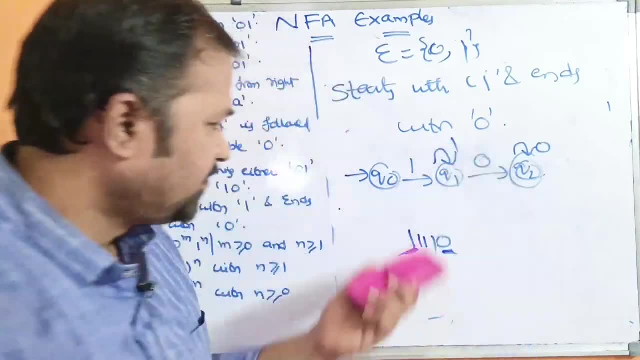 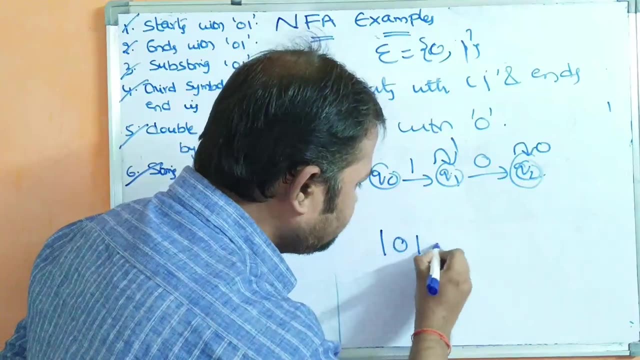 in between 1 and 0, we can have any number of 1s, So let us apply 1.. If we apply 0, then we will go to the Q 2 state, And here we may have a situation like this: 1 0,, 1 0. So 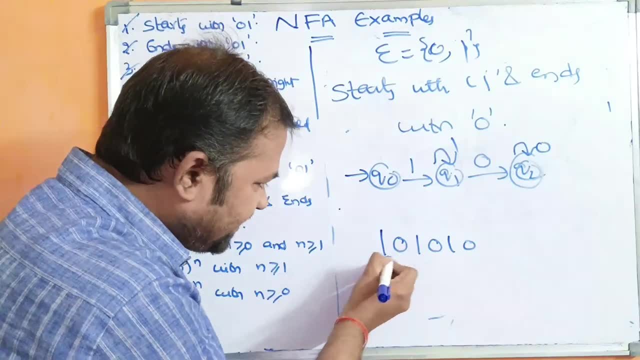 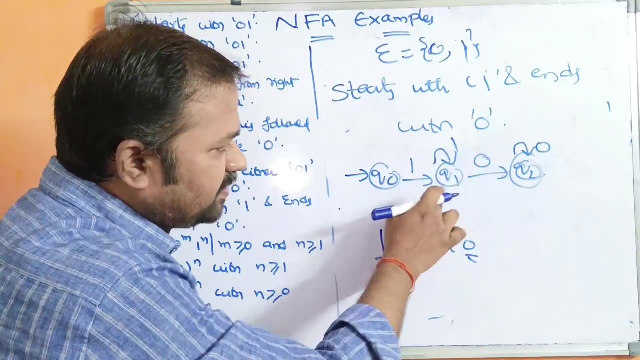 1 0,, 1 0,, 1 0.. So here the string is starting with 1.. Ends with 0.. So if we apply 1 on Q naught, we will move to the Q 1 state. If we apply 0 on Q 1,. 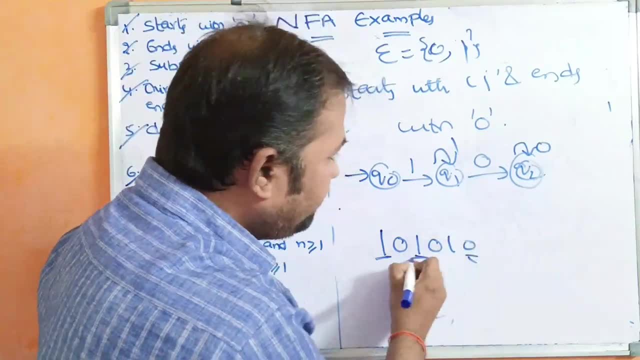 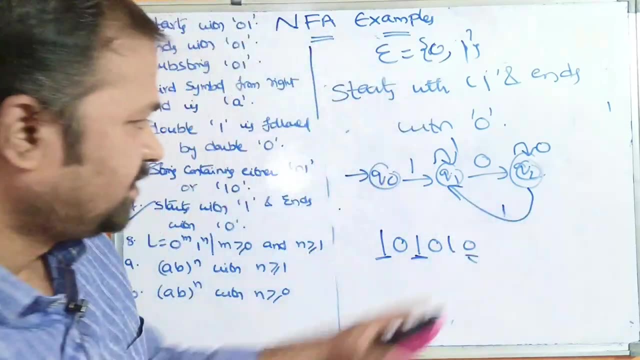 we will move to the Q 2 state, And after that we have to apply 1 on Q 2.. So, likewise here, let us apply 1 on Q 2.. So we will move to the Q 1 state. We will move to the Q 1 state Next. 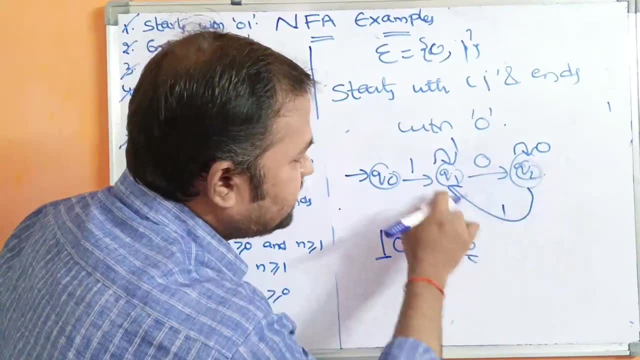 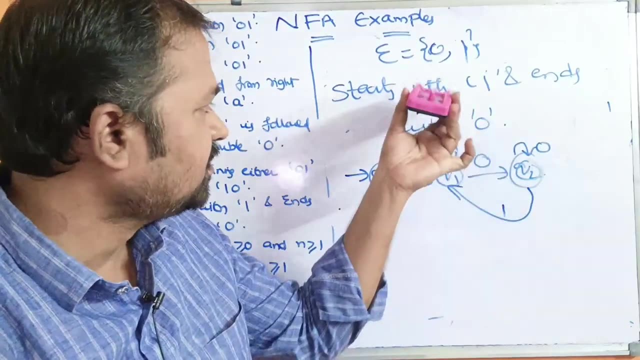 let us apply 0. So 0. Q 2 state. Next, 1: 0.. So Q 2 will be the final state. So in this way we can solve the problem. Okay, So this is NFA for the strings which starts with 1 and ends with 0.. Okay, Now let us see the 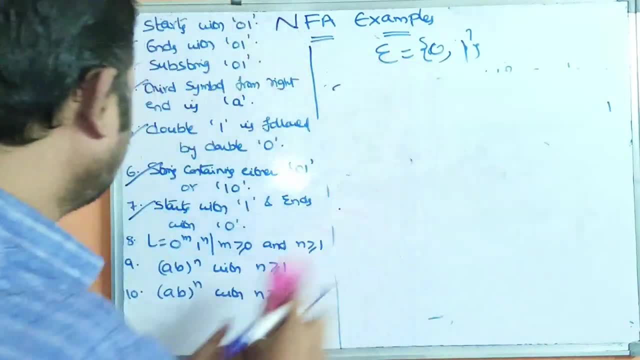 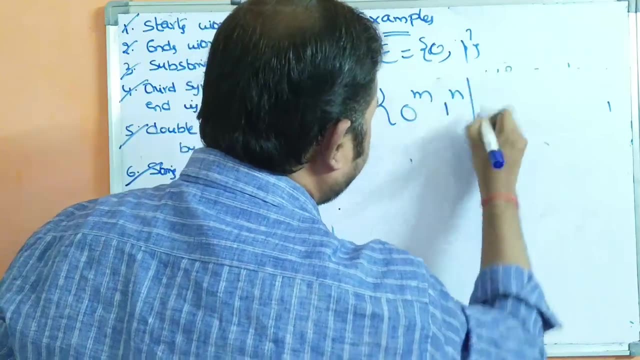 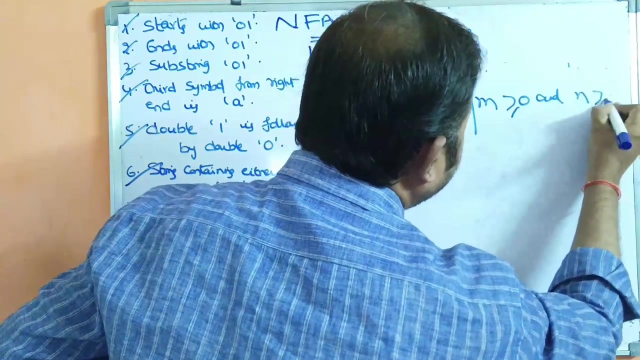 remaining three examples. So L is equal to- here directly the language is given. So L is equal to 0 power m, 1 power n, such that m is greater than or equal to 0 and n is greater than or equal to 1.. m is greater than or equal to 0, whereas n is greater than or equal to 0. 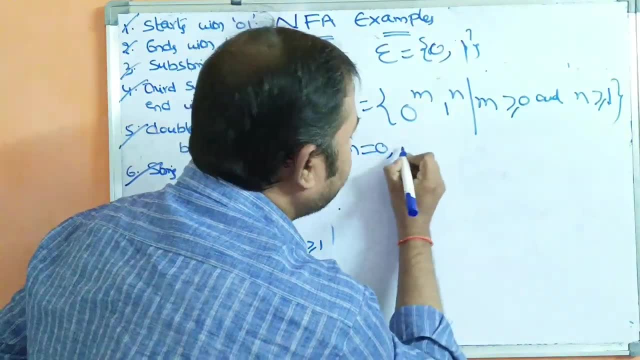 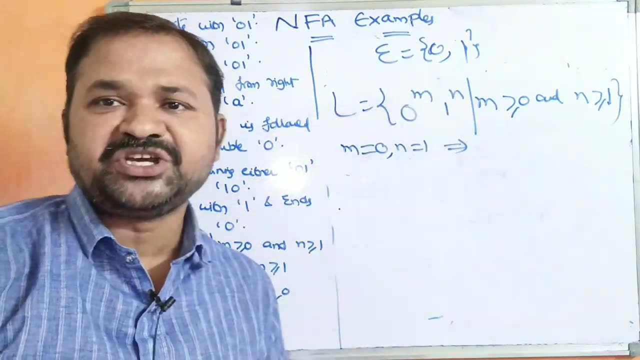 greater than or equal to 1. let us consider m as 0, n as 1. then what is the string here? 0 power. m means 0, so 0 power. 0 means 0. number of zeros. next, 1 power n. n value is 1, so 1 power 1. 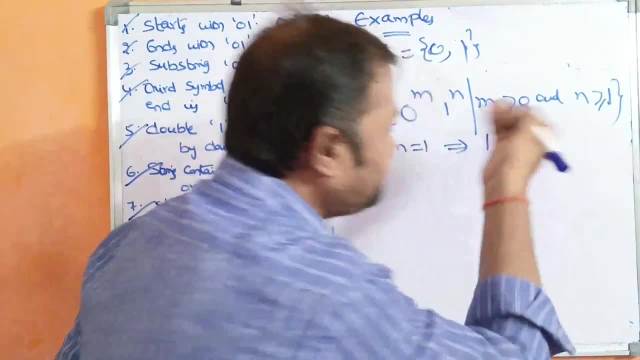 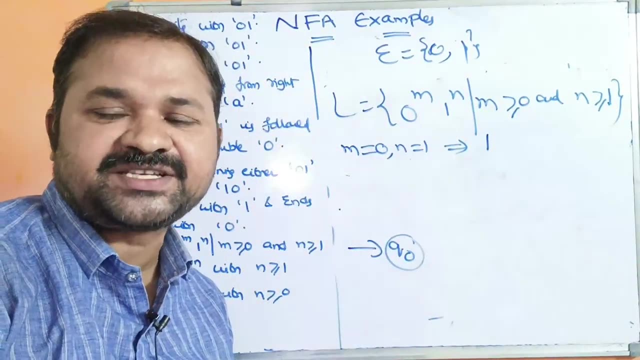 means single 1. okay, so here the string is 1. okay, so if we apply so, here the string length is 1. so 1 means we require how many states? 1 plus 1, two states, so q naught q1. so if we apply 1 on the. 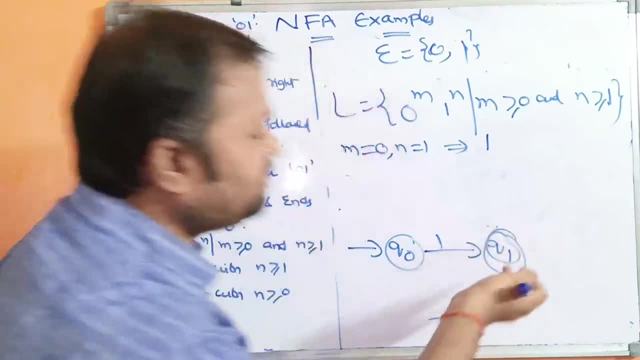 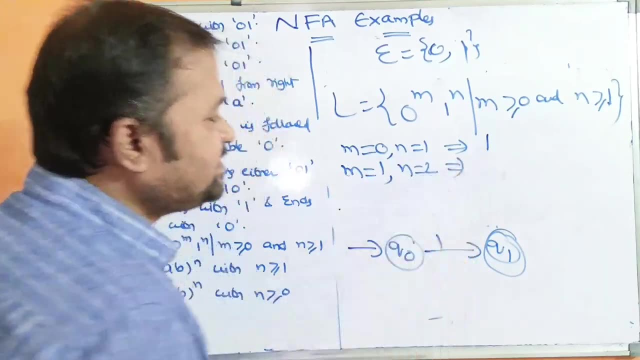 q naught, then we will move to the q1 state. so this q1 is the final state. now let us take one more scenario. let: m is equal to 1, n is equal to 2, m is equal to 1, n is equal to 2. so 0 power 1. 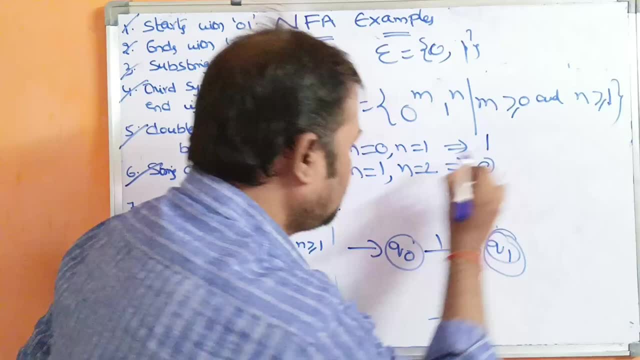 so 0 power 1 means single, 0, n is equal to 2, that means 1 power 2. 1 power 2 means two ones. so 0 power 1 means single, 0, n is equal to 2, that means 1 power 2. 1 power 2 means two ones. 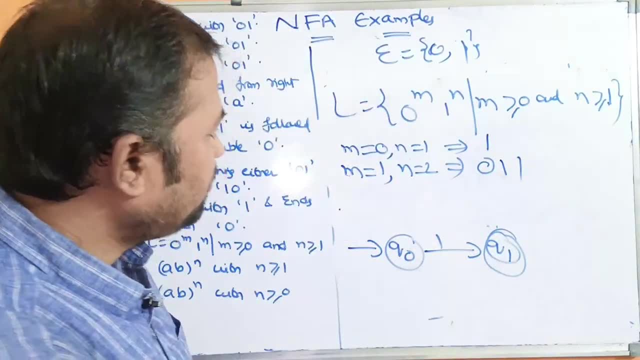 so 0 power 1 means single, 0 n is equal to 2, that means 1 power 2, 1 power 2 means two ones. so 0 double 1, 0 double 1. okay, so here we have 0 double 1. so we, if we apply 0 on q naught, then we: 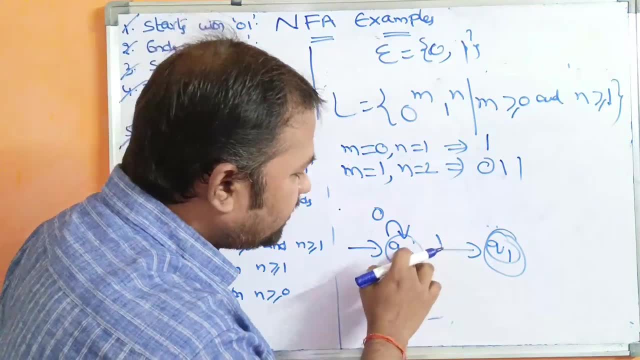 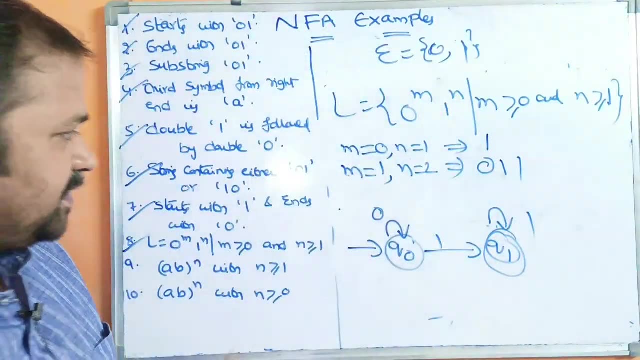 will be at q naught state only. if we apply 1 on q naught, we will move to the q1 state. next, if we apply 1 on q1, then we will be at q1 state only. okay, let us take one more scenario and check. 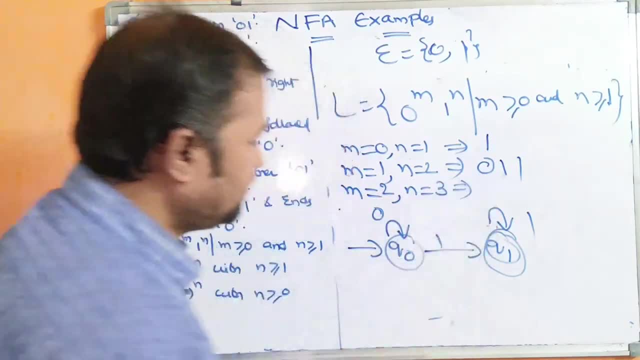 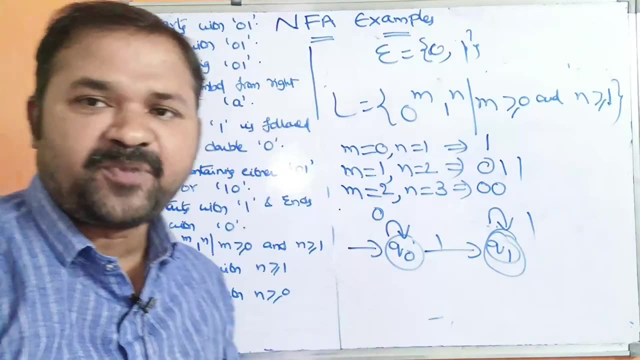 whether it is correct or not. m is equal to 2, n is equal to 3, so m is equal to 2, means 0 power. 2, that means 2 zeros. n is equal to 3 means 1 power, 3, 1 power. 3 means 3 ones, 3 ones. so apply 0 on q. 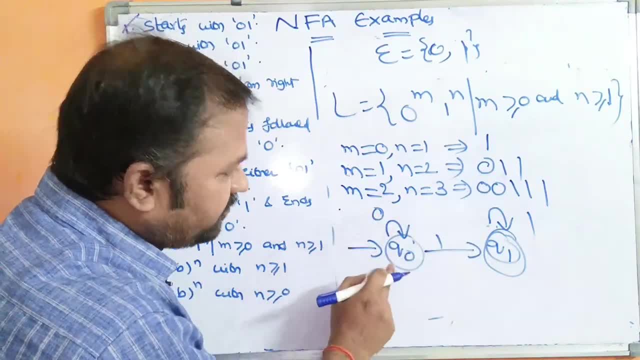 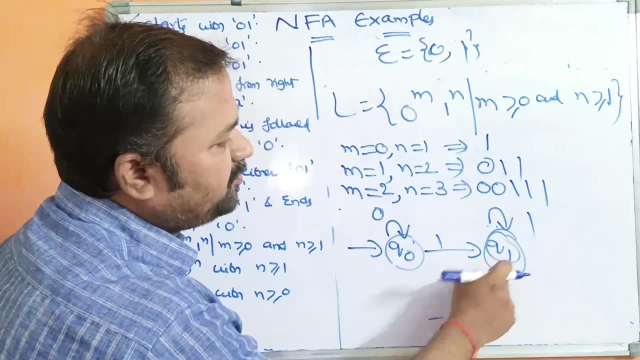 naught: we will be at q naught only. apply 0 on q naught: we will be at q naught only. apply 1 on q naught: we will move to the q1 state. apply 1 on q1: we will be at q1 only. apply 1 on q1: we will be at. 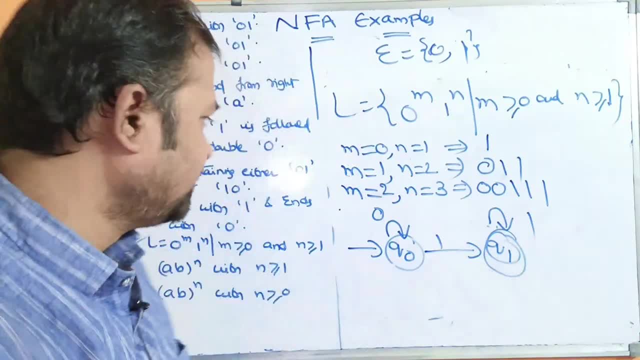 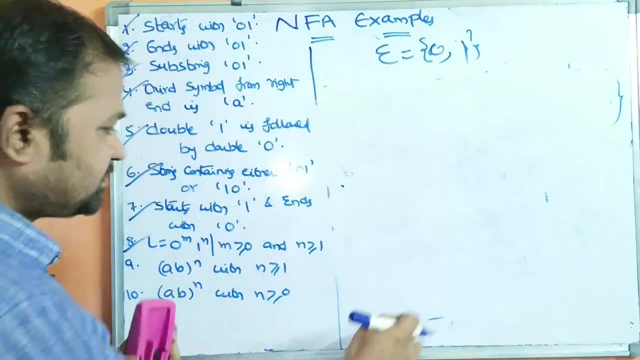 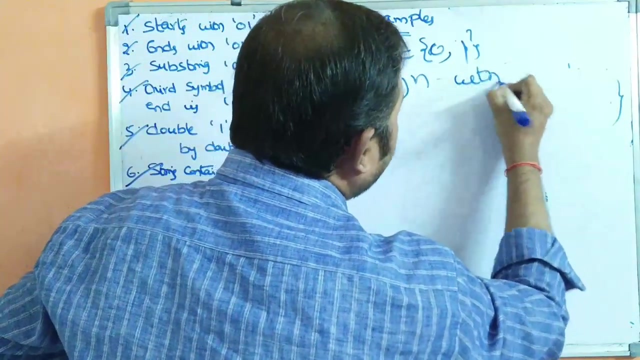 q1, only q1 is the final state. so this is the value string. now let us see the next problem. so what is the next problem? here? also, some expression is given, some language is given ab whole power. n with n is greater than or equal to 1 with n is greater than or equal to 1. ab whole. 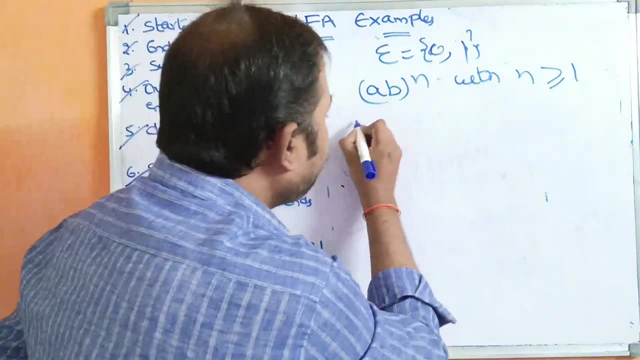 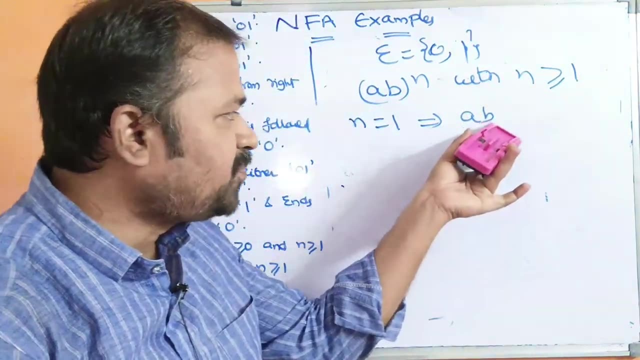 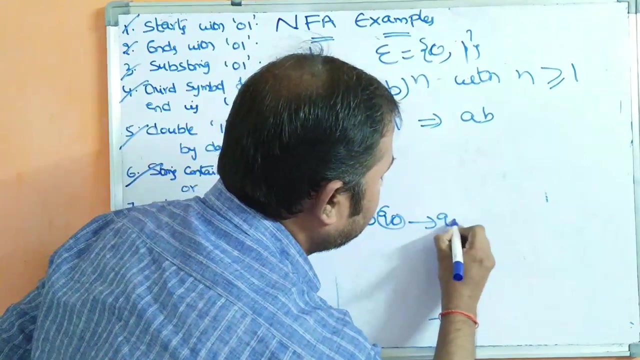 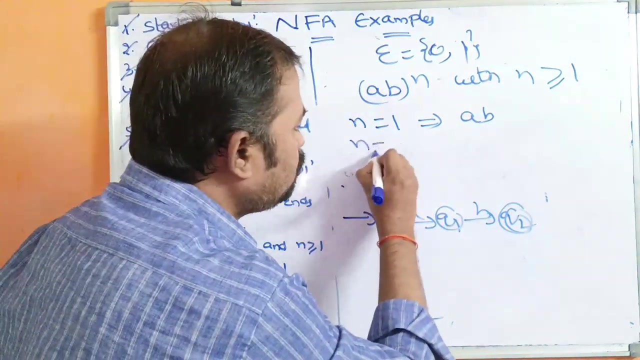 power n with n is greater than or equal to 1. so if n is equal to 1, then what is the string? ab? whole power: 1. so that is nothing but ab. so here the minimum possible string is ab. so ab means length, three states. so q naught q1, q2, so q2 is the final state, ab, okay. next, if n is equal to 2, then ab, ab. 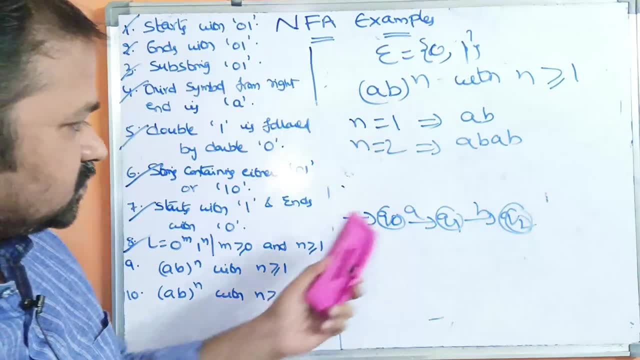 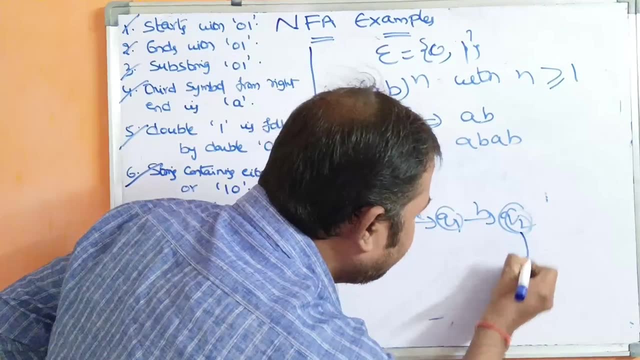 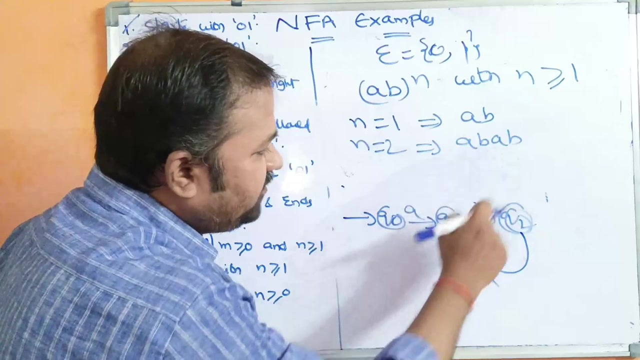 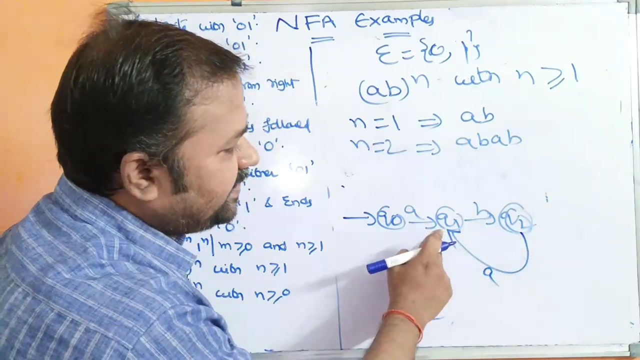 ab, ab, so ab, ab. okay. so next here, a is applied here. next b is applied here. next, let us make a transition like this: so if we apply a and q, naught, we will move to the q1 state. if we apply b and q1, we will move to the q2 state. next, if we apply a and q2, we will move to the q1 state. if we 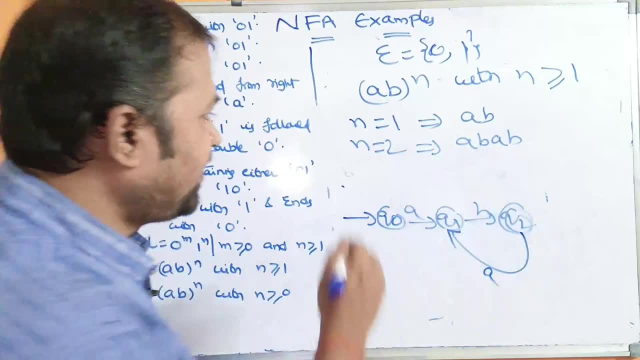 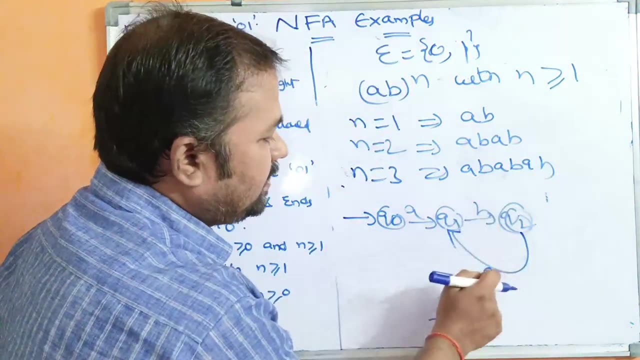 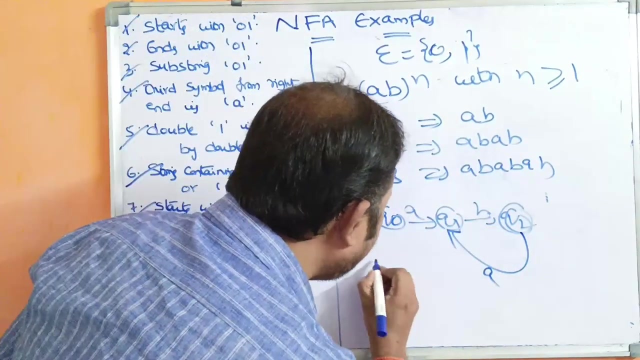 apply b and q1, we will move to the q2, so q2 is the final state. likewise, if n is equal to 3, ab, ab, ab. so ab, ab, ab. so this is the finite automata. in this way we can construct. let us see the last. 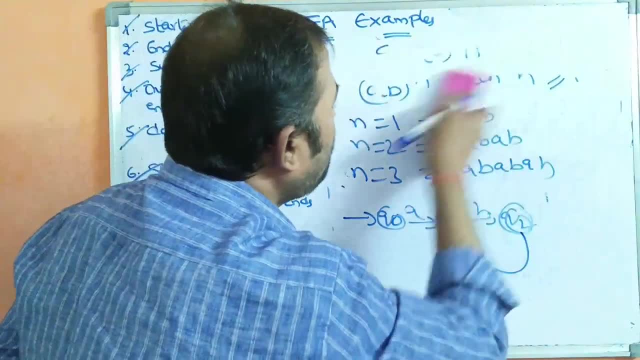 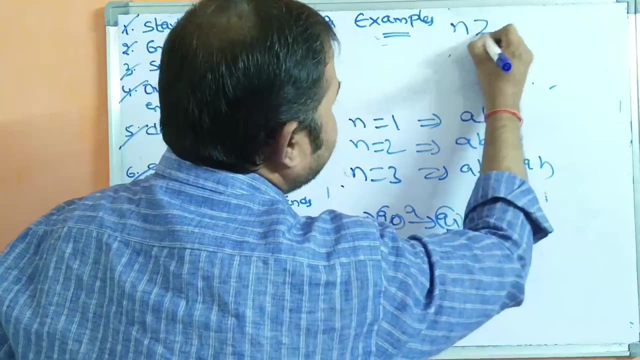 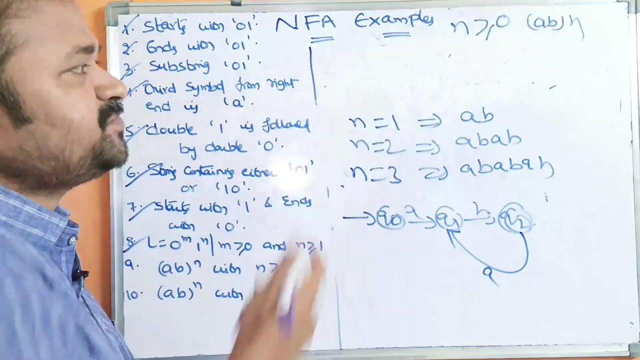 example. the last example is ab whole power n. whole power n with n is greater than or equal to 0, with n is greater than or equal to 0. ab whole power n. whereas in the previous problem n value is 1, but here n is starting from 0 onwards. so if 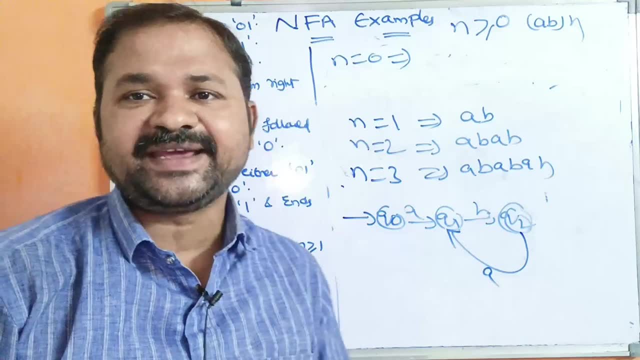 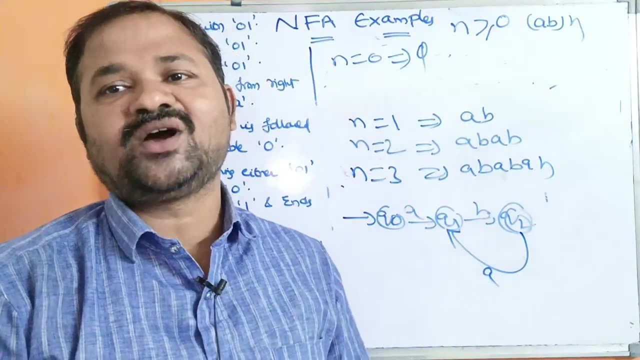 n is equal to 0, then ab whole power 0 is nothing but empty string. it is empty string, so some pi symbol empty string. so that means the initial state should also becomes final state. okay, why? because without applying any symbol also we have to get the final state. okay. 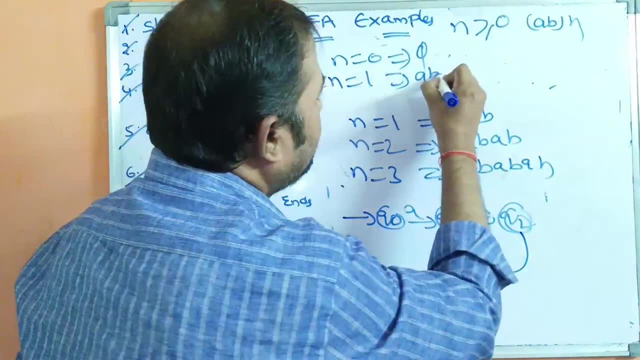 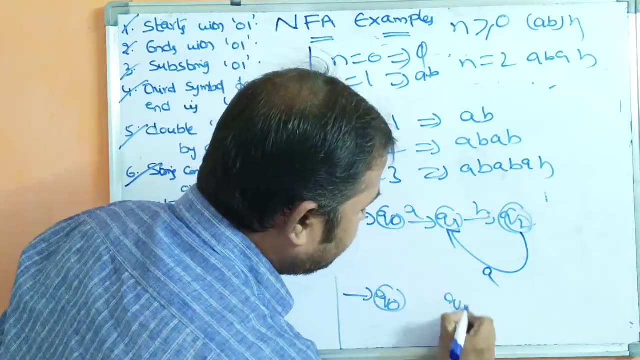 next, if n is equal to 1, then same ab. if n is equal to 2, then ab, ab. so let us draw the diagram. so q naught, q1. here, the both the states are final states. q naught is the final state, as well as q1 is. 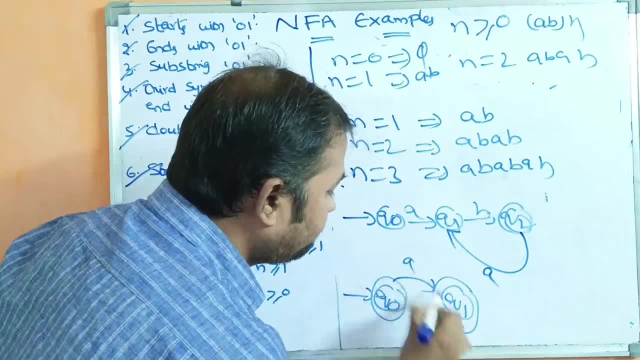 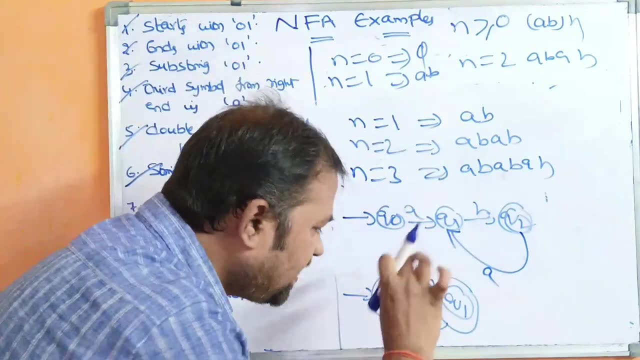 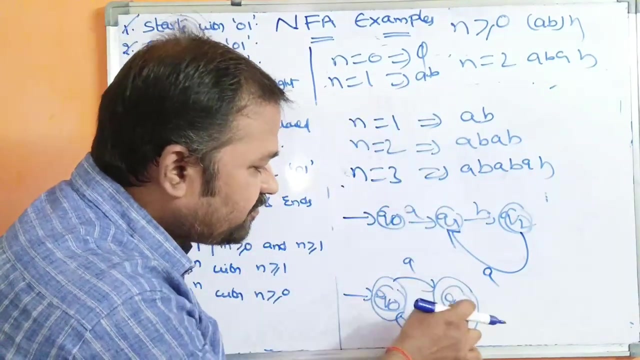 also the final state. okay. so let us apply a here, b here, okay. first one is: n is equal to 0. that means here we did not apply any symbol, but we are at the final state. only the initial state is the final state. okay. next ab. so if we apply a and q, naught, we will go to the q1. next, if we apply b and q1, we 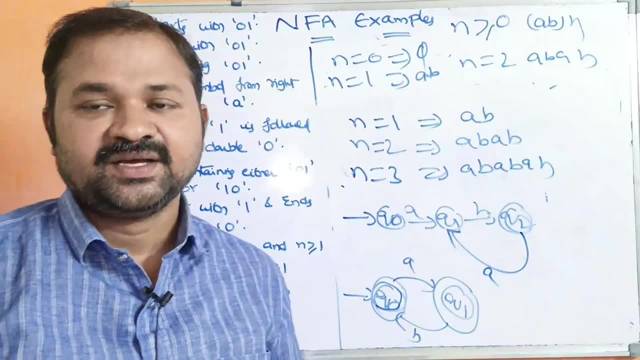 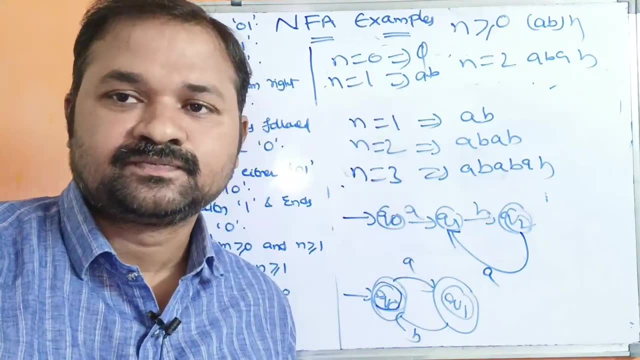 will move to the q naught. so q naught is nothing but final state. okay. so in this way we can solve problems by using the nfa. so this is about nfa examples.